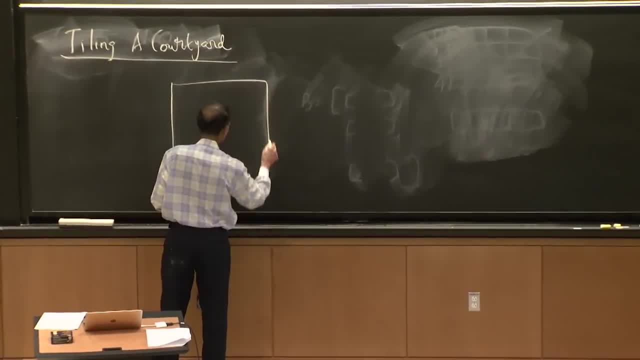 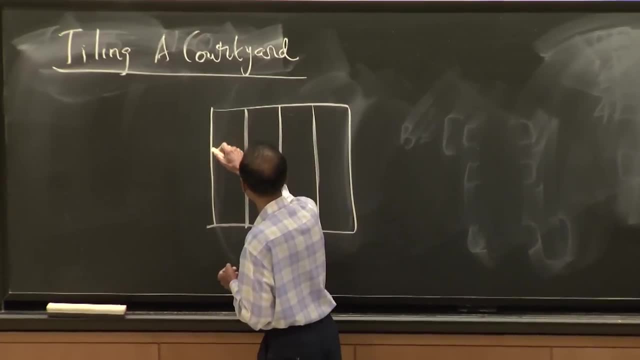 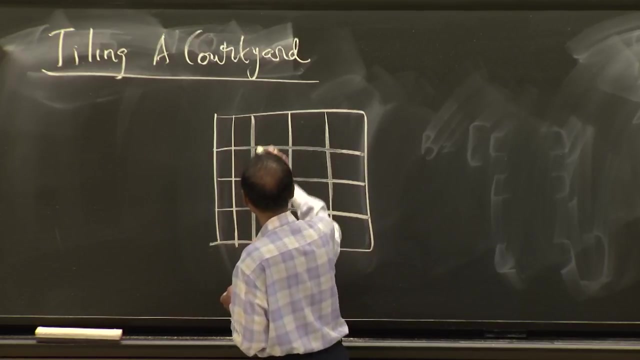 But I'll set up the puzzle. I guess I didn't have to erase it. I'll erase this square. It's a courtyard that has a bunch of its tile. You're supposed to tile it And it's all square tiles And I'll just make it 8 by 8, like a chess board. 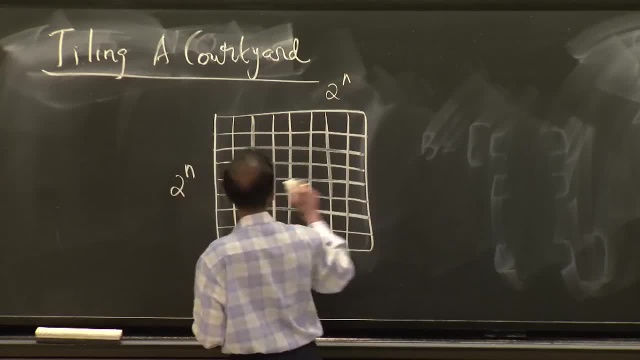 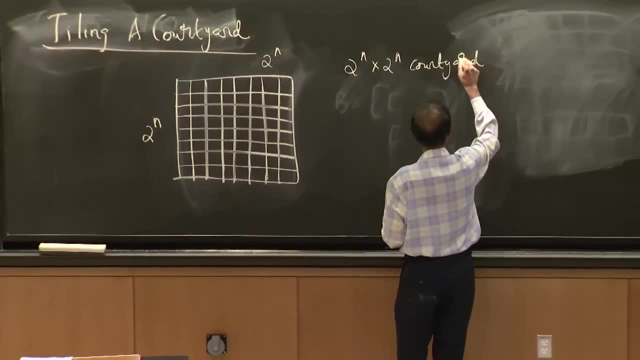 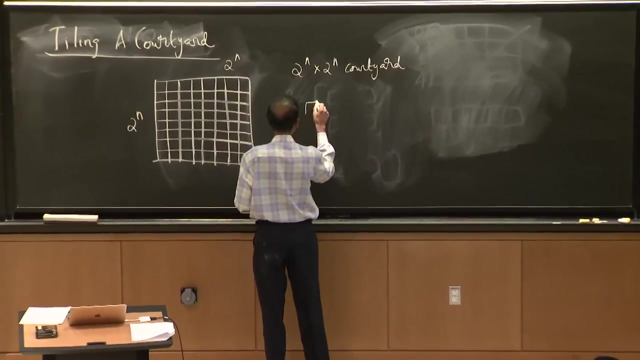 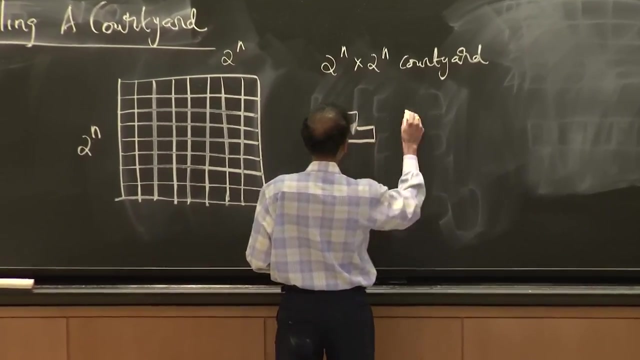 And in general, we're going to say that this is 2 raised to n By 2 raised to n- courtyard, All right, And I want to tile this courtyard. So this is a three-tile. Some people call it a tromino. 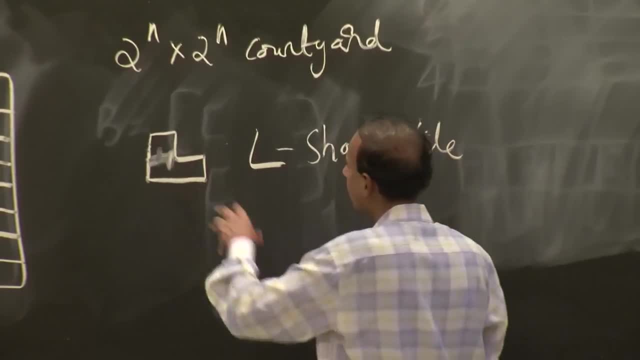 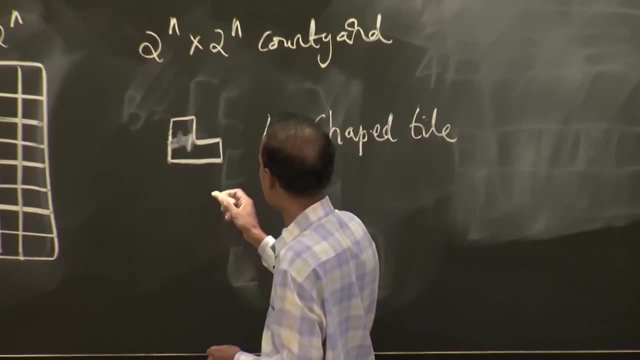 You can think of it as really an L-shaped tile And it can be oriented. It can be oriented in any different way. I mean, it could be an inverted L, et cetera, And you're supposed to tile this courtyard using L-shaped tiles. 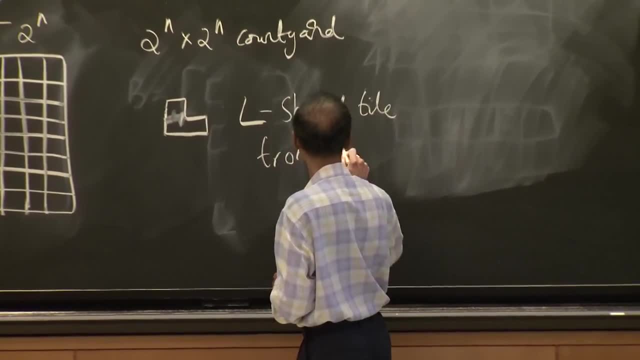 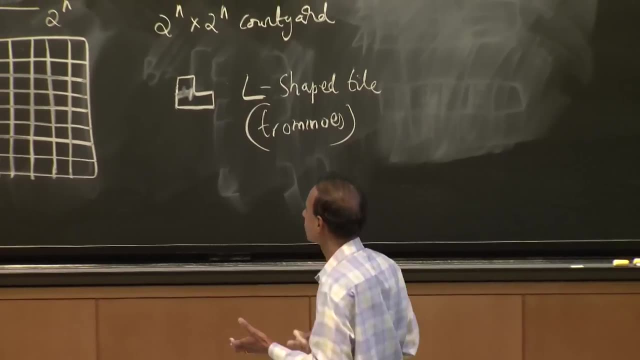 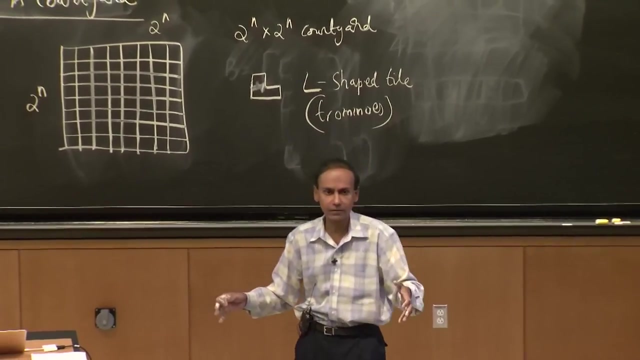 or trominoes, And they call it trominoes because there's three tiles in there, three squares in there, And so that's your job, right? I guess kind of a weird job, but this is a puzzle, And so you're out there. 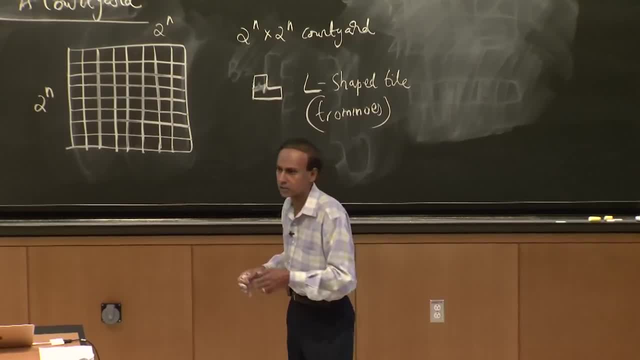 It's 2 raised to n by 2 raised to n, And all you have are these L-shaped tiles And you're not allowed to break them. I mean, if you break them, then that's not considered a valid tiling. 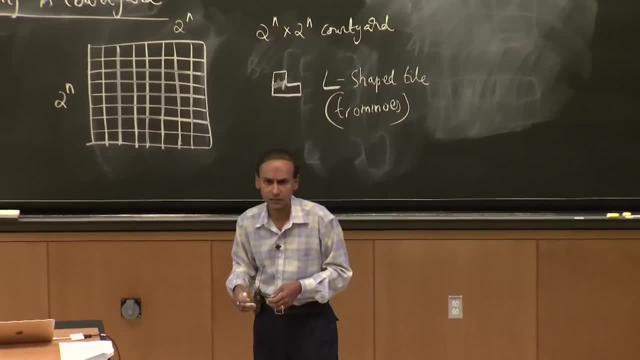 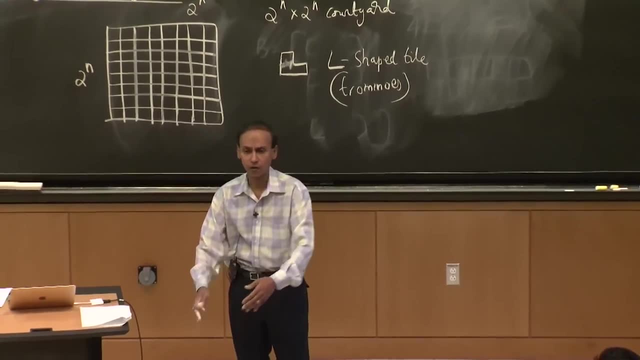 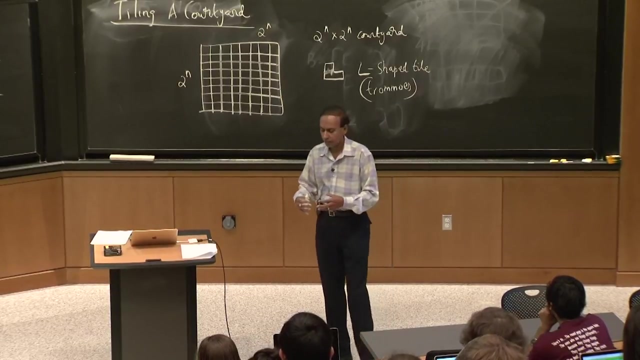 That's bad And that's your job, right? So is this a Oh? and obviously it needs to look like this. It needs to look like the floor. Maybe you're allowed to see the markings, because these are tiles after all. 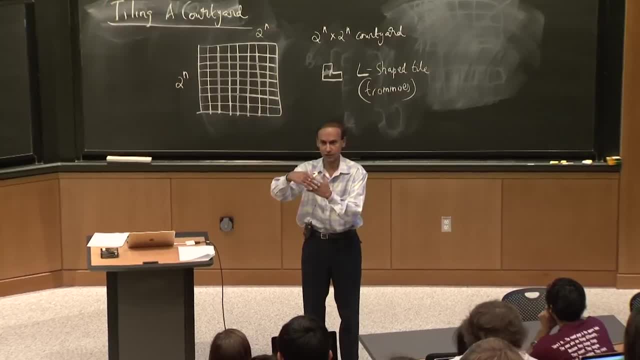 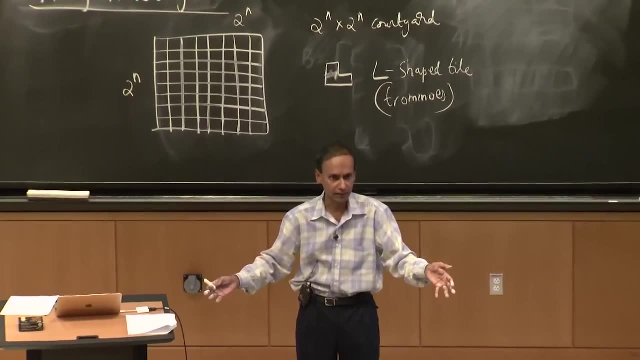 But you can't have something that is uneven, You can't have a tile on top of another tile. I mean that's a definite no-no, And you can't not have a tile in any part of the courtyard. So I think that was kind of obvious. 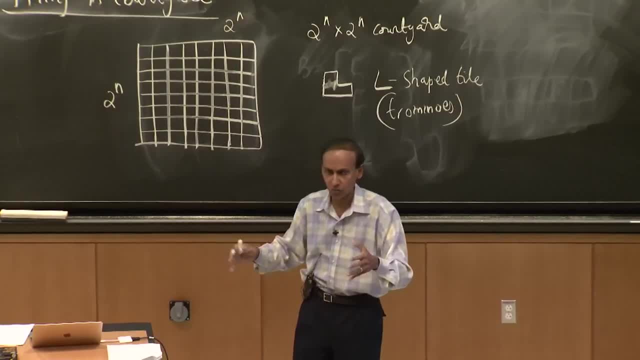 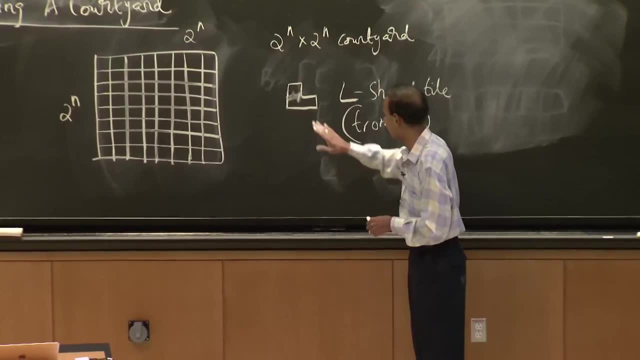 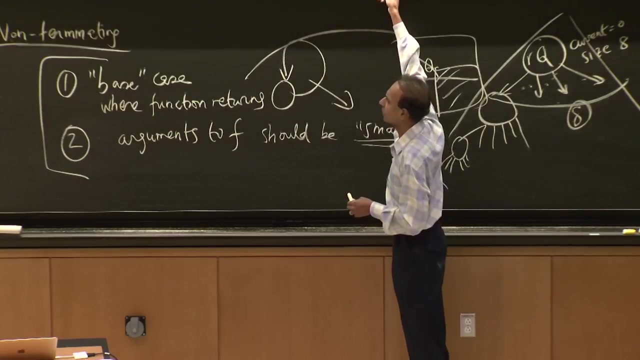 But it's worth explicitly stating, just so we don't get confused here. So that's the question that we're going to try and answer, But, as I said, I want to talk about, I think, something a little bit different, for about 5 or 10. 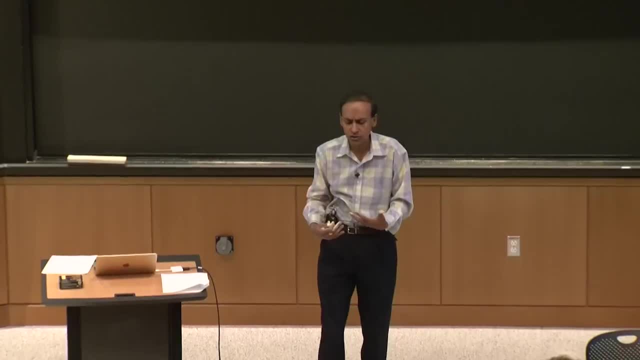 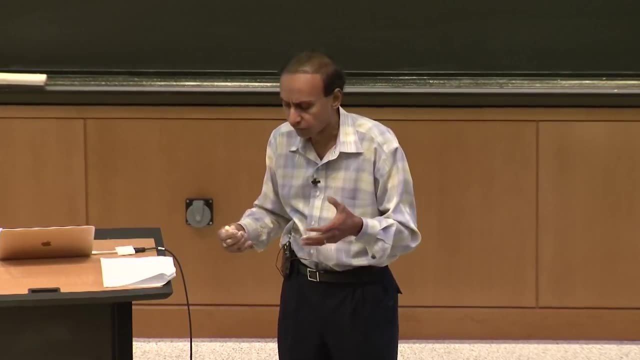 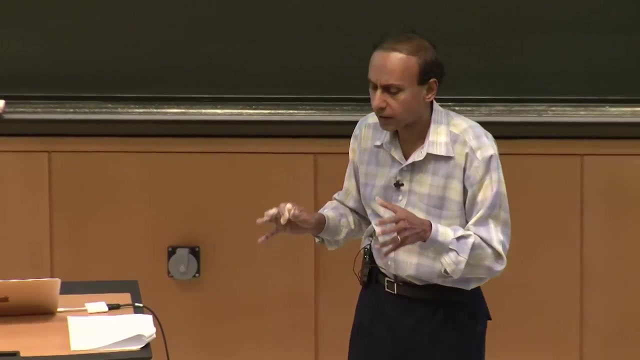 minutes and actually show you some code, Because I want to introduce this notion. that's a little bit different from the N-Queens recursive paradigm. It is recursive, But it's called recursive divide and conquer. all right, And usually when we use the term recursive divide, 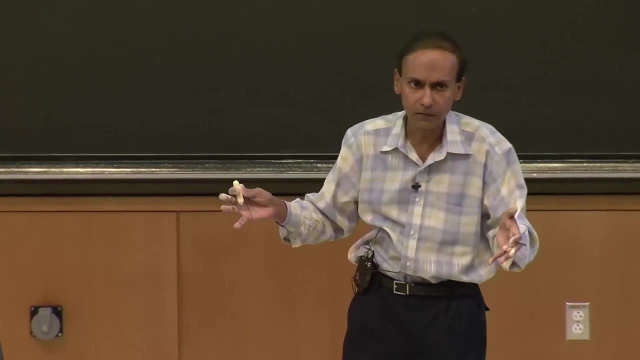 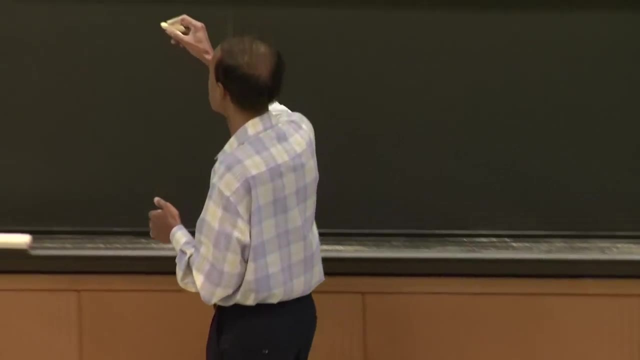 and conquer. you might think that it's applicable even to the N-Queens recursive code, But it fits. It fits From a technical term standpoint. when we say recursive divide and conquer, we're really saying that we're taking the problem. 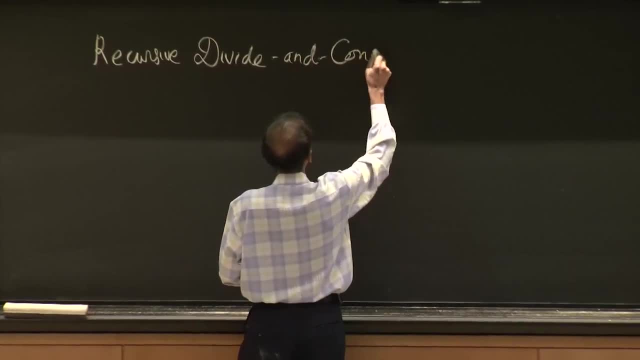 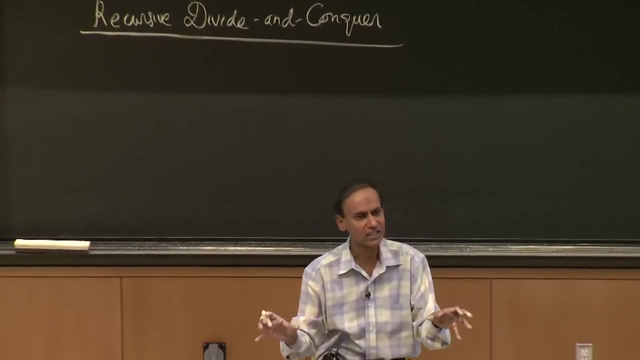 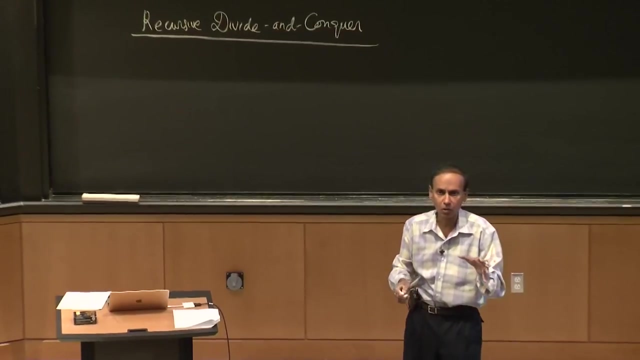 and we're dividing it up into smaller problems. So you take the problem and you divide it into two problems that are half the size, or three problems that are a third of the size, et cetera, which is not what happened in the case of the N-Queens. 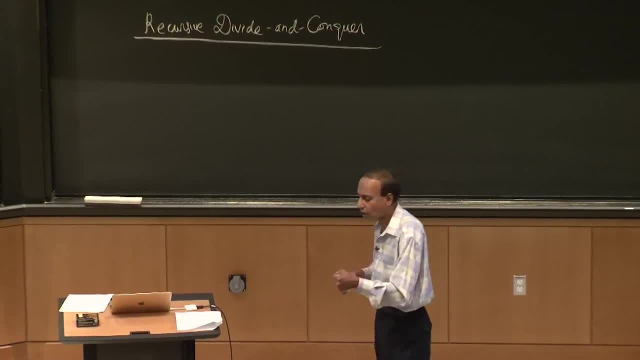 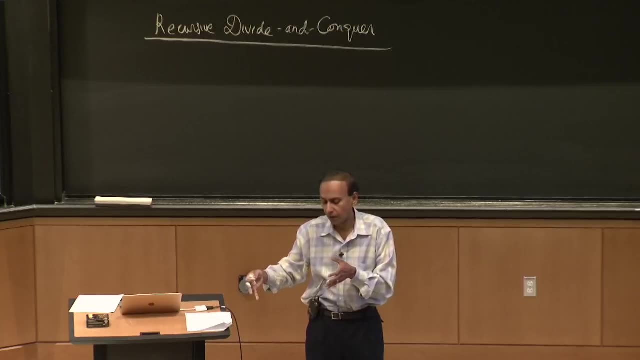 problem, right? I mean, in the case of the N-Queens problem, you took a column and you actually did iterations on the column so that it potentially exploded on you, And then you had a problem that was slightly smaller than the N-Queens. 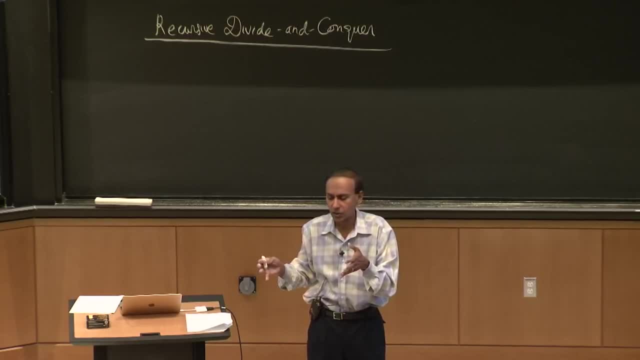 It was effectively N minus 1 Queens right, And so it's not N over 2 or N over 2, or three N over 3s in the case of a three-way recursive divide and conquer. So there's a qualitative difference. 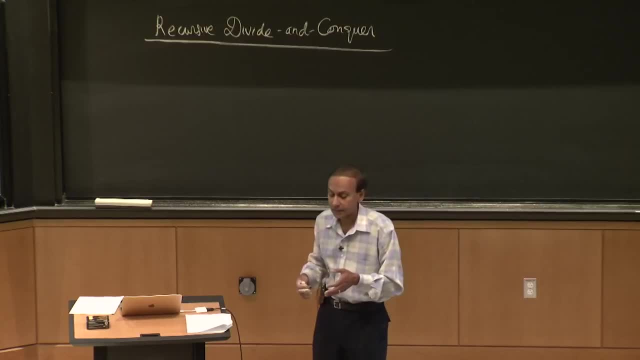 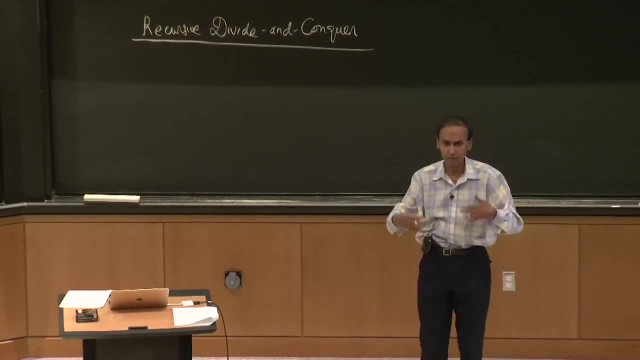 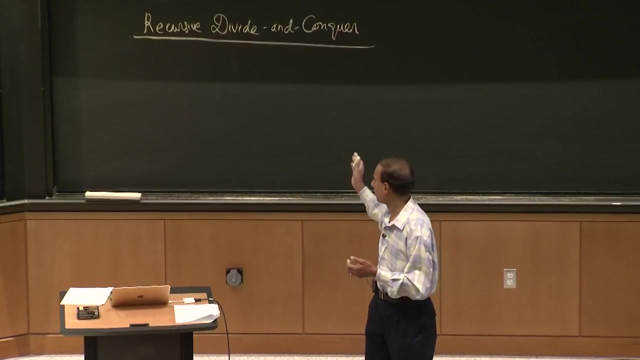 And there's also a quantitative difference in the sense that these kinds of algorithms are going to be efficient in that they're going to run very quickly in polynomial time, perhaps quadratic time. We can do some analysis for both the merge sort that we're going to do now and for the tiling puzzle. 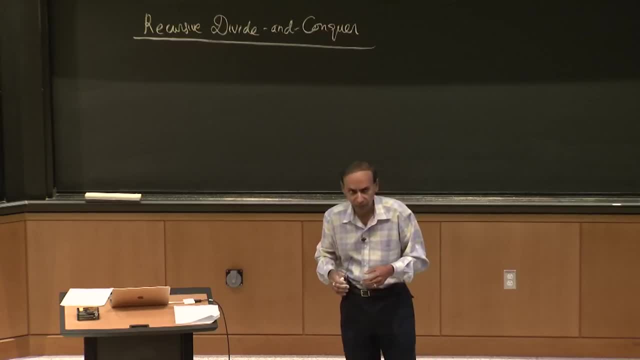 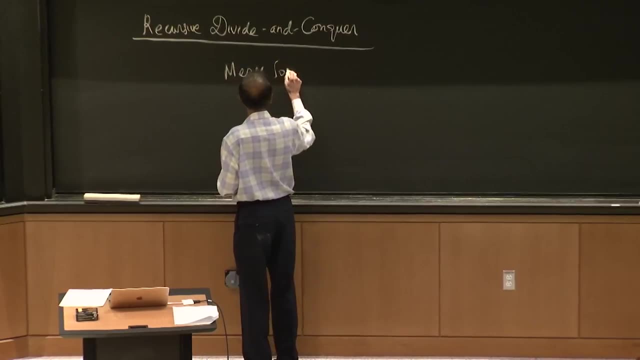 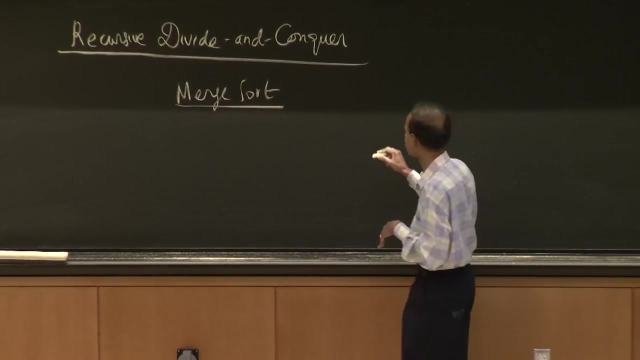 once we get to that. But that's something to keep in mind, all right. So merge sort is the canonical recursive divide and conquer approach And I'll put up code for it, but I'm not going to show it to you. You can look at it in the website. 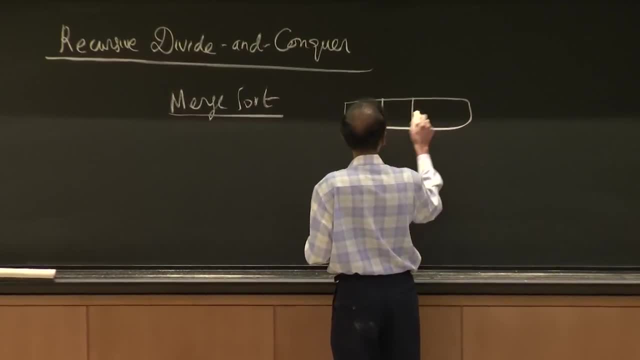 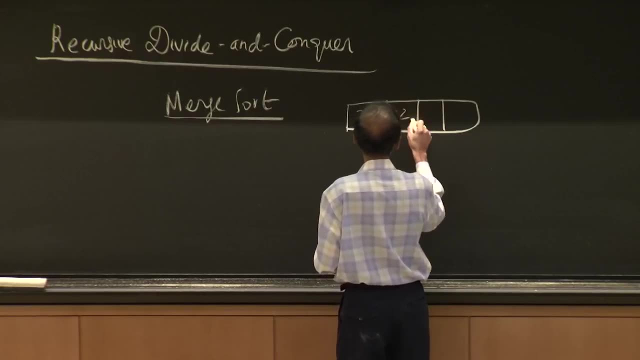 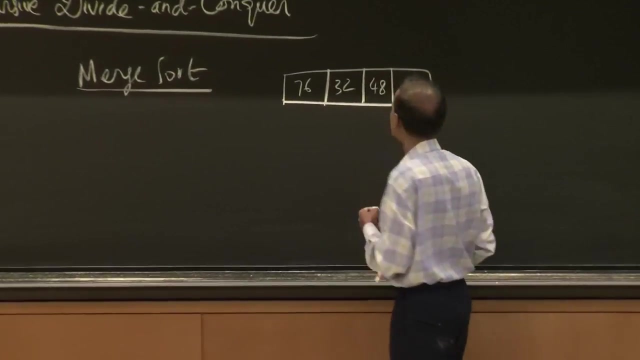 But I'm going to describe the algorithm to you using a trivial example, And so I want to sort these numbers in ascending order. All right, So I have these four numbers that I want to sort in ascending order, And obviously I could do this many different ways. 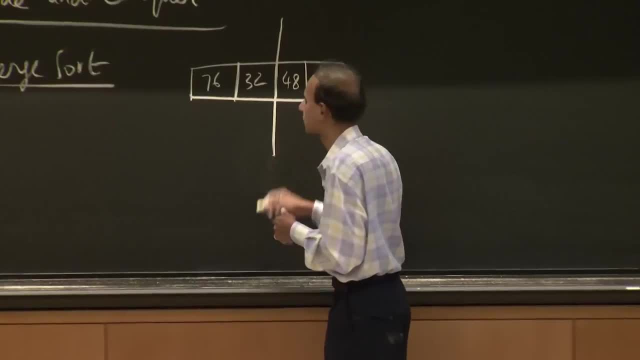 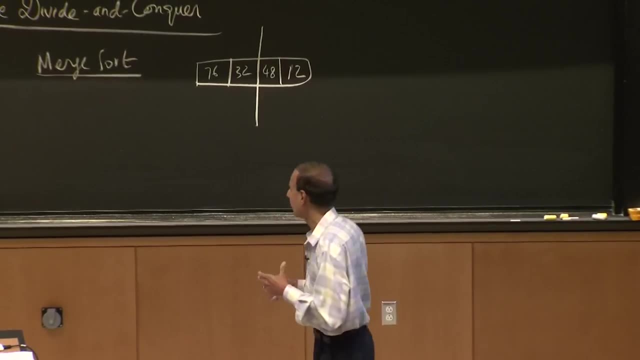 We looked at selection sort, But this is a large array And I want to do something more efficient than a quadratic algorithm, an n-squared algorithm And merge sort, which is recursive, divide and conquer fits the bill. And what merge sort says is I'm going to split the array. 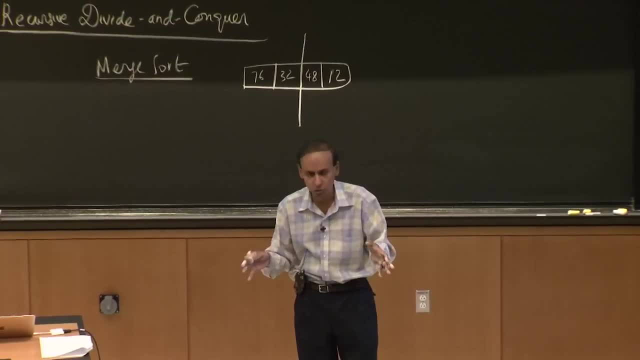 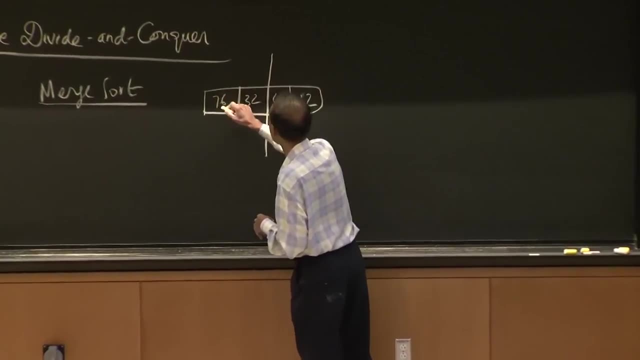 I'm just going to take this array and I'm going to split it up into two sub-arrays, And I could do this recursively, But let's just talk about the first step, right? So I'm going to go ahead and split this array up. 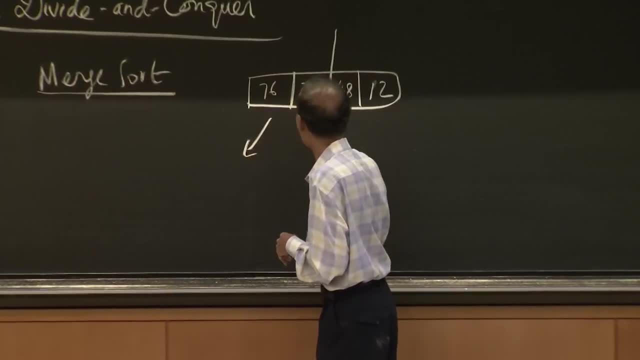 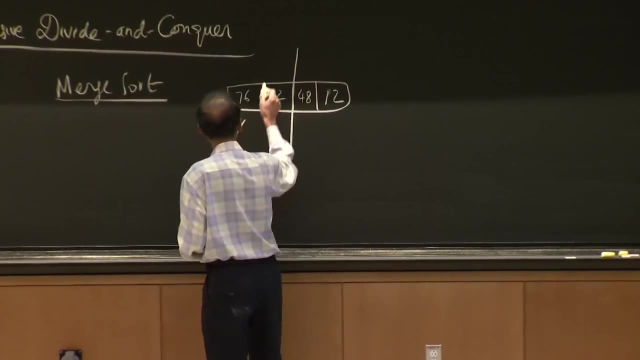 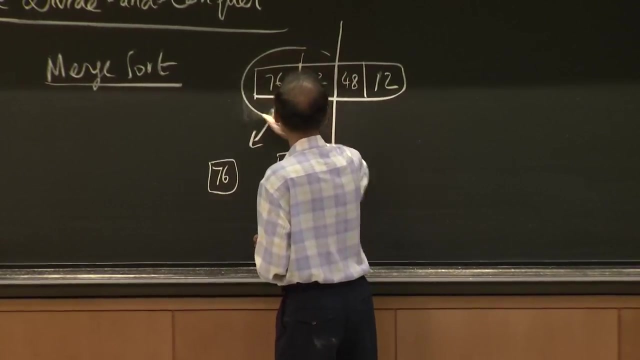 And I have 76 and 32.. And I'm going to call merge sort on this smaller array And the first thing that that merge sort does is split the array up into something smaller And you end up getting that. So this is the first thing. 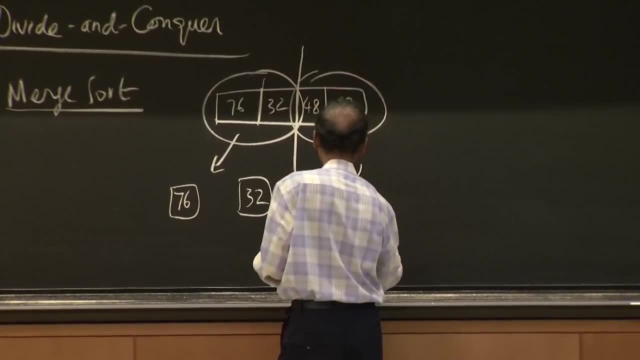 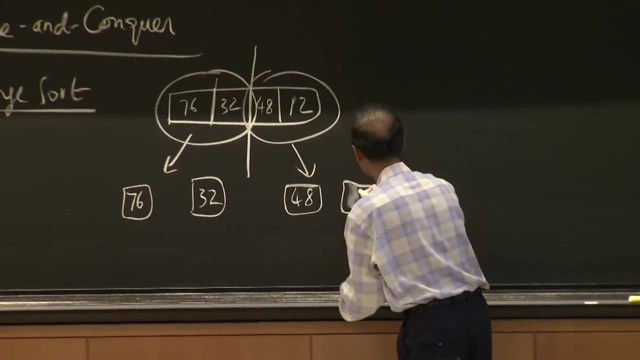 And that's the first split. And then you end up splitting 48 and 32.. And, I'm sorry, 12.. 76, 32,, 48,, 12.. Yep, I got that right And so far you've done nothing. 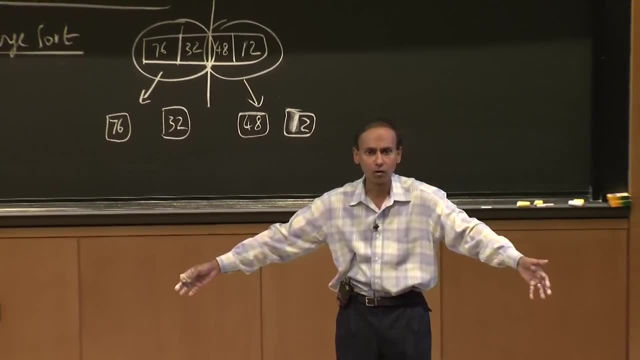 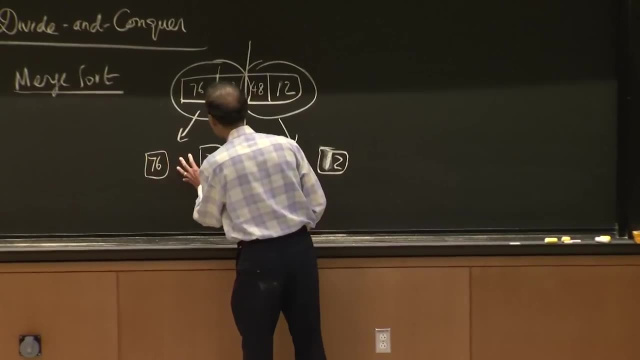 I mean, you've just sort of broken things up and turned this into four, one arrays or one list or what have you right? But then the fun starts where, after you do the split, after you return, and so 76, a singleton is trivially sorted. 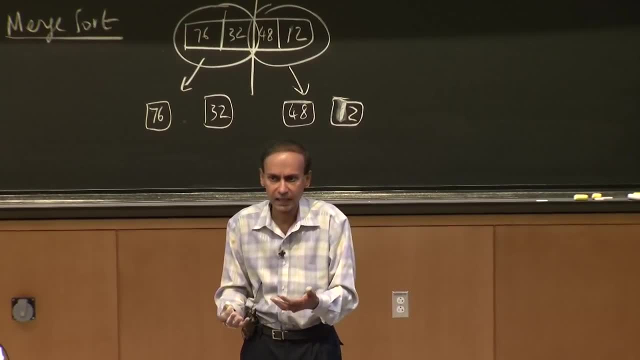 So there's no work to do. So there's no more splits that you could do. There's nothing that says you can't. I mean 76 is a monolithic element in the array, So you can't do anything with it. 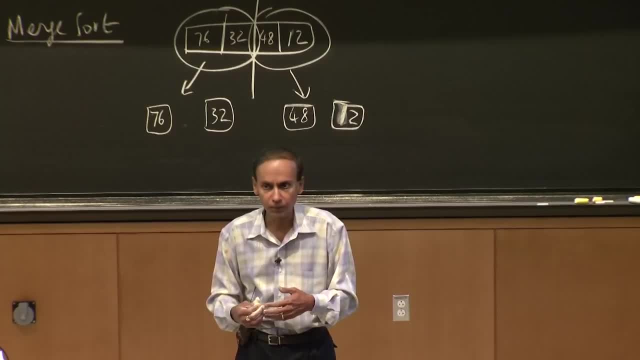 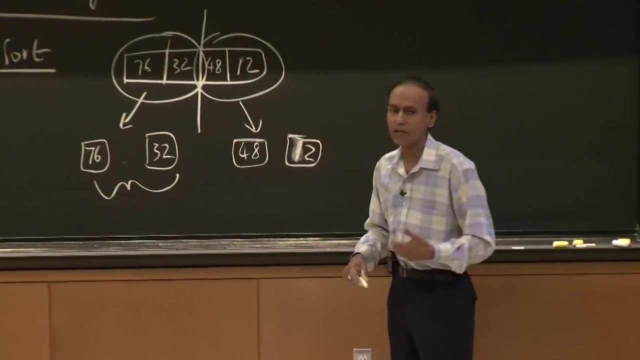 And so you just leave it be, And the same thing with 32 and so on and so forth. But after your two calls return, you have to merge the two together. right, And the way you merge the two together, the invariant here is that when you merge the two together, 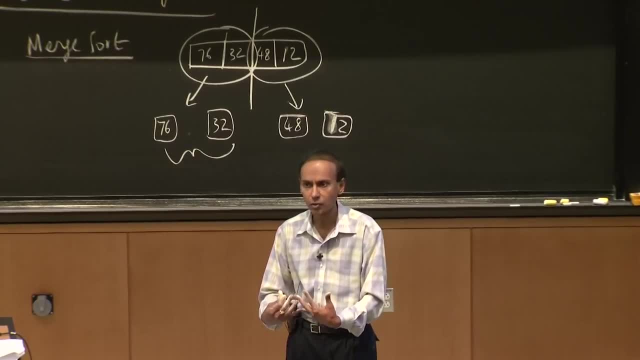 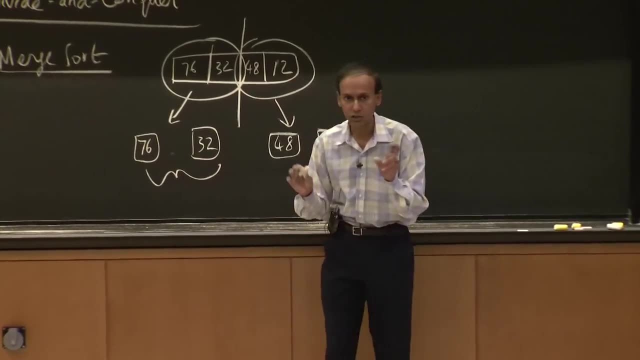 they have to be sorted in the order that you want the overall array to be sorted, which is ascending order, right? So in this case, down at the bottom, it's trivial code because you have two singleton lists And you just decide which order they go into. OK, 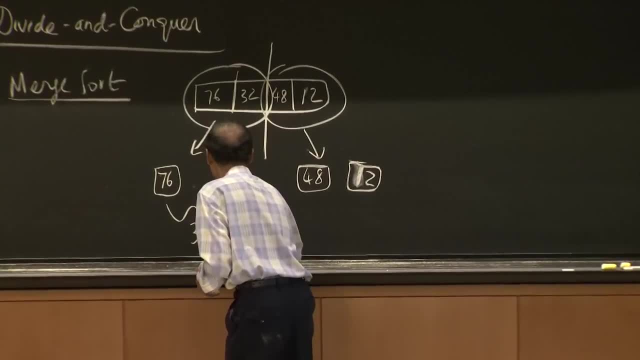 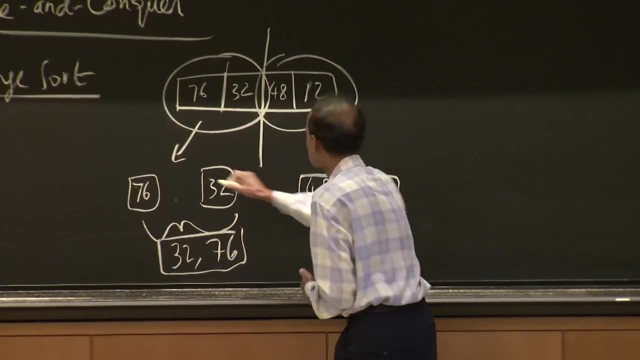 So the merge in this case would simply produce 32 and 76,. OK, And in this case the merge would produce 12 and 48,. all right, So at this level you're going to return 32 and 76 back. 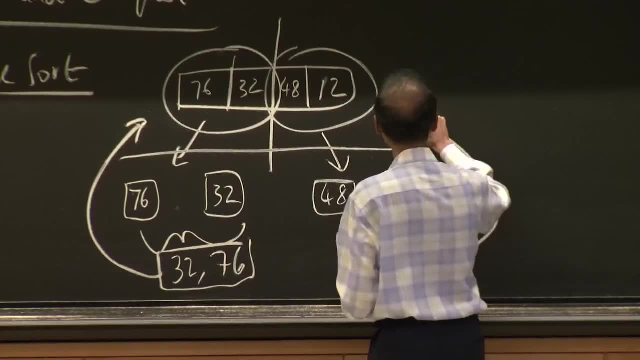 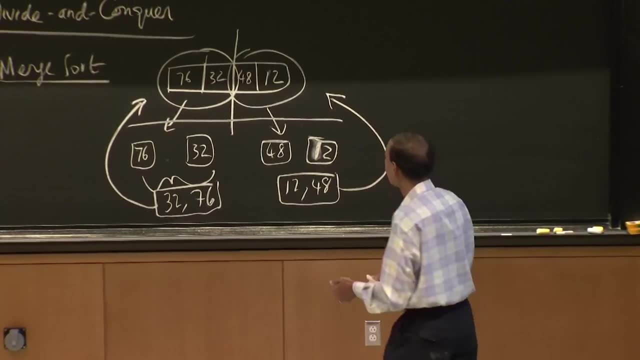 You're going to return 32 and 76 back, And here you're going to return 12 and 48 back. OK, Now it gets a little more interesting. OK, Now it gets a little more interesting because now you have 32 and 76 and 12 and 48. 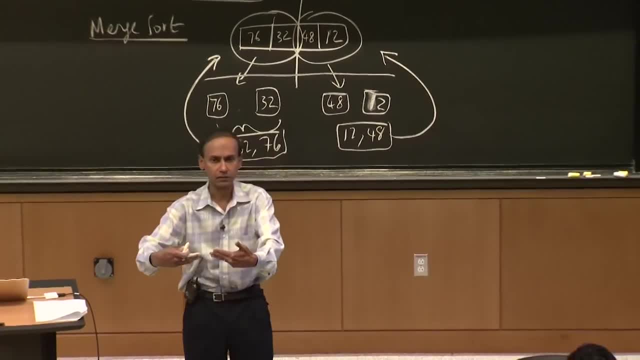 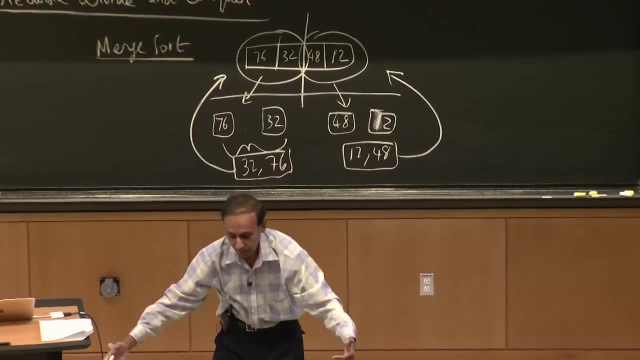 And those are both sorted in ascending order And you need to merge them together, right And so if you had a 128-element list, you would go all the way down And then you would do some merging, come up all the way. 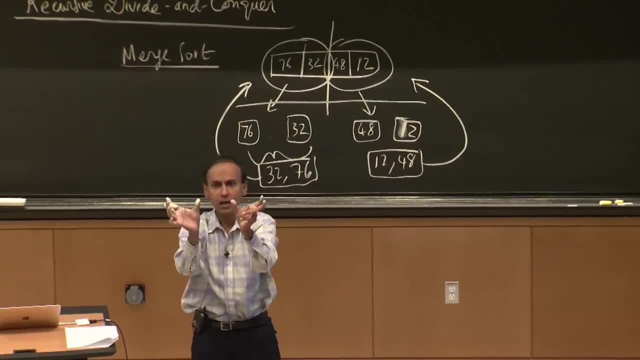 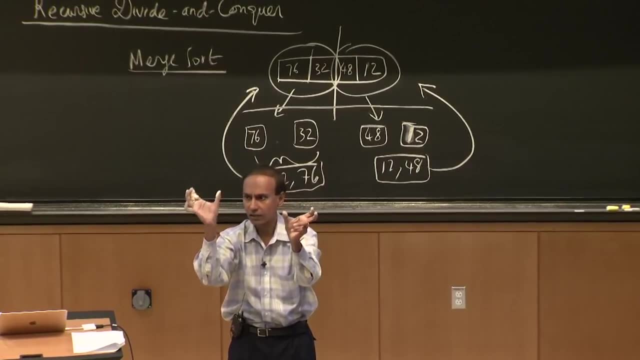 And then the most time-consuming step really would be taking two 64-element lists that the left one is in ascending order and the right one is in ascending order, And then you need to merge them together, so the result is in ascending order, right. 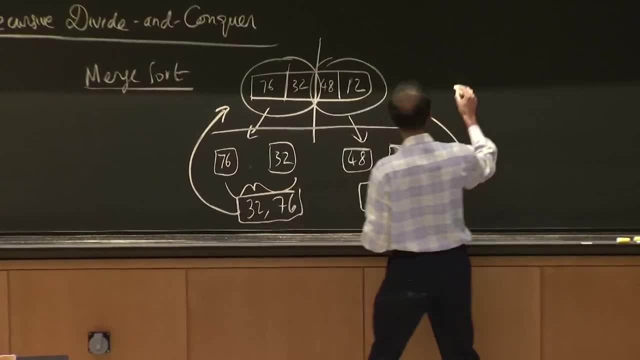 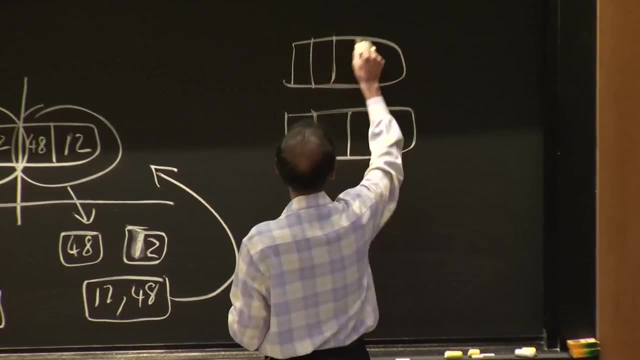 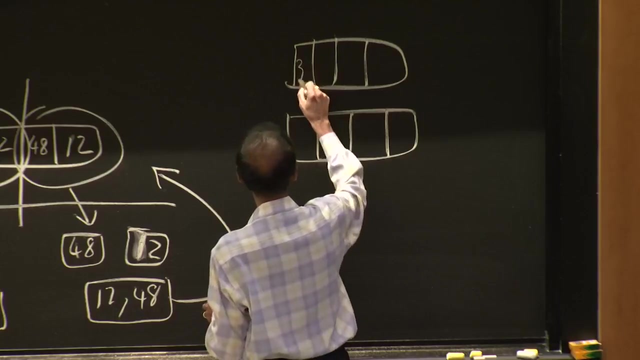 Does that make sense, And so, in this case, the way we're going to do this is, if you have- and I can do this for this example or a different example, But you know what, I'll just stick with- 32,, 76,. 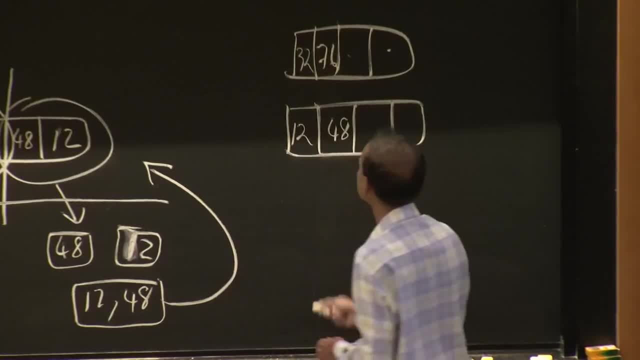 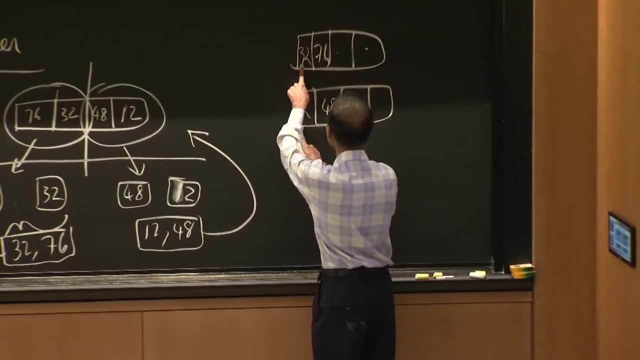 and this could be larger. This is 12 and 48. So I need to merge these two to produce an ascending order, And we use a straightforward algorithm that's called the two-finger Two-finger algorithm, which says I'm going to start with my fingers pointing. 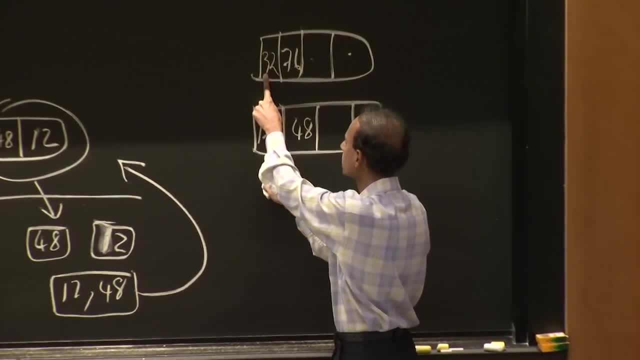 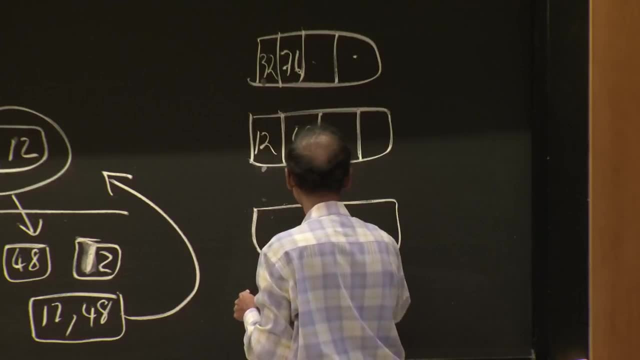 to the beginning of the two arrays And I'm going to choose the element that's smaller And I'm going to write it into my output array, right? So I'm going to compare 32 and 12.. 12 is smaller, so I'm going to write 12 down. 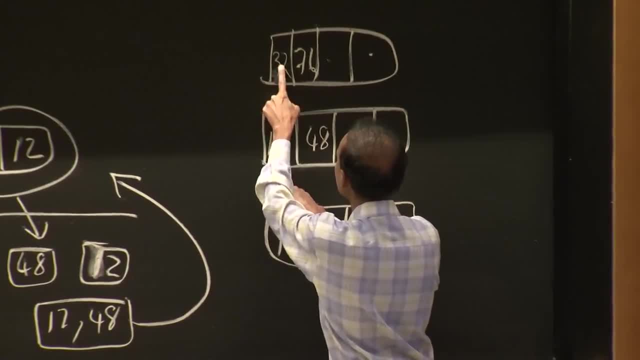 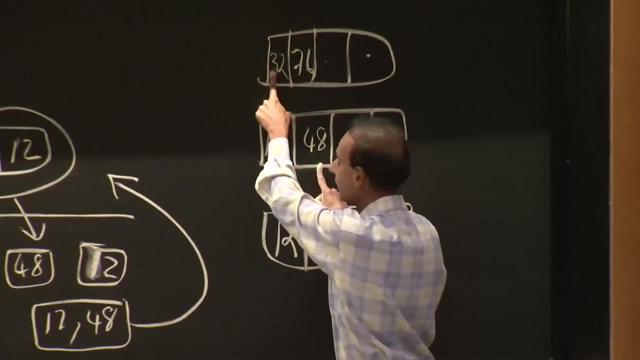 And because I picked 12 from this array and I didn't pick 32, I'm going to leave my top finger where it is And I'm going to move my bottom finger, my right-hand finger, over to the next element, right? 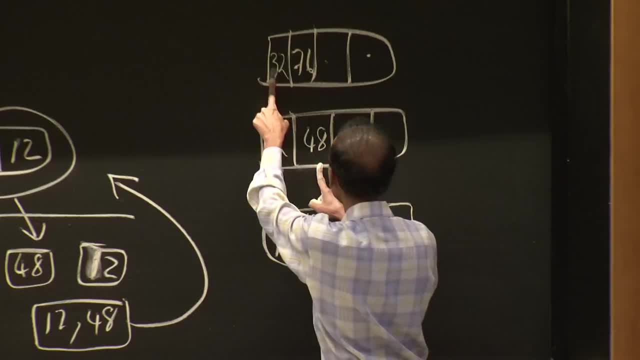 And then I'm going to compare 32 with 48, because this finger didn't move- And I'm going to figure out which one is smaller And it's 32.. And I'm going to put that over here And then I'm going to move this finger. 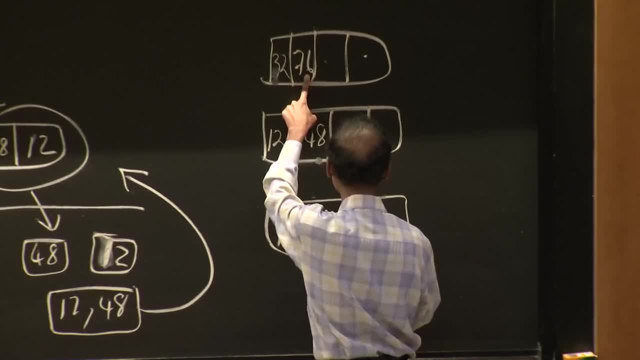 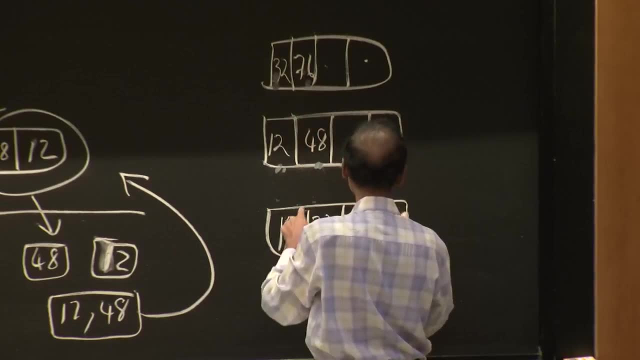 because I took away 32.. And then at this point 48 is smaller, And then I'm off this array, assuming the array ended here, But if it didn't, I keep going. And then the last thing I do is put 76 down. OK, 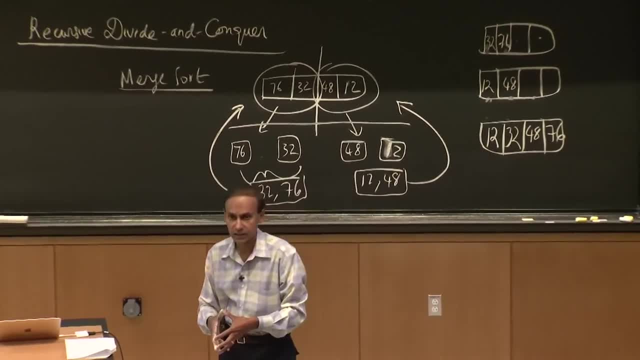 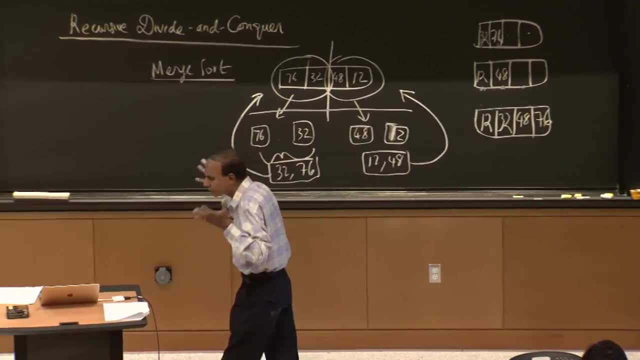 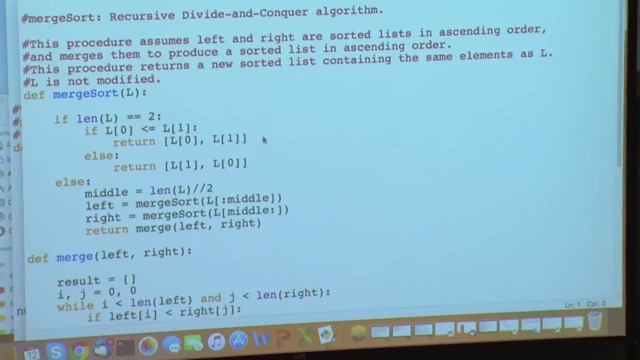 So that is a recursive divide and conquer algorithm, right? It's the simplest algorithm I can think of. that is still interesting And I'll show you code for it. I'm not going to explain it, But it's worth looking at the overall code. 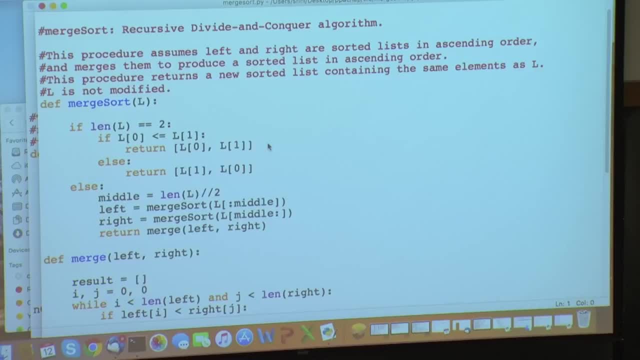 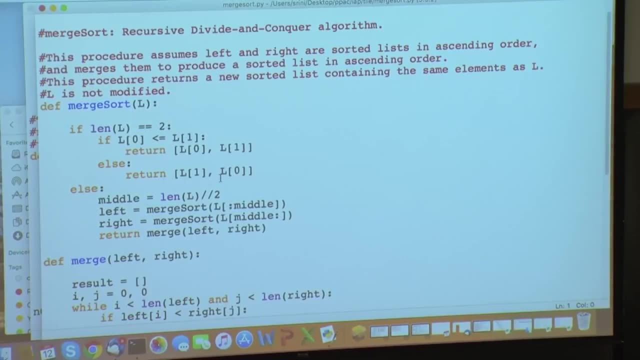 And then the merge, which is this two-finger algorithm, is actually the most amount of code, But the split itself, as you can see, is, you see, as with our recursion, we say we want to have a base case, And so when the length of the list 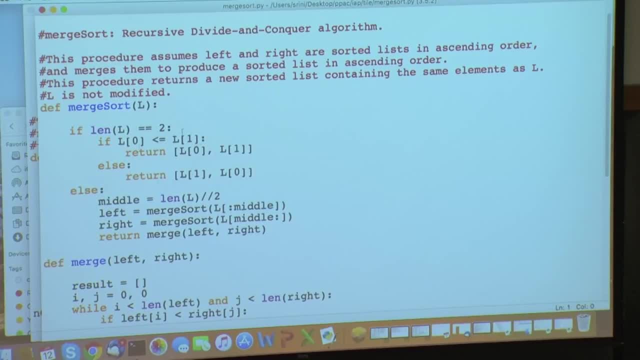 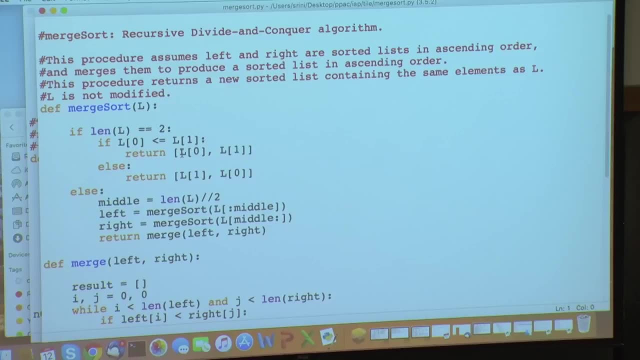 becomes 2,. I'm just going to do that little flip. This is a sorting algorithm that only works for a list of length 2, right, But the beauty of this is that I can keep going down to get smaller and smaller lists, such that the sorting algorithm 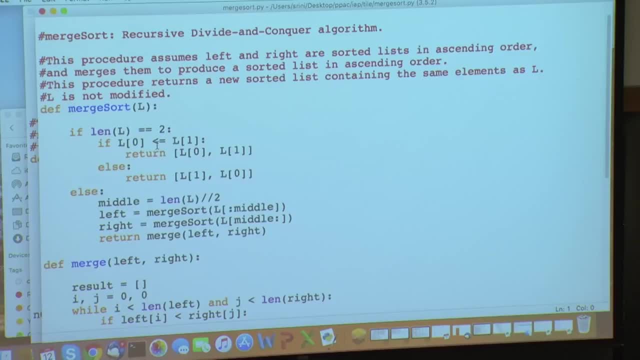 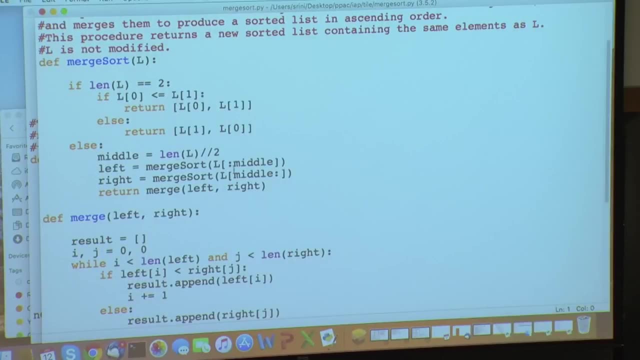 actually works, And this is it. This is a fine sorting algorithm for a base case, right, And we do have a base case here. We also have the other property that I'm actually calling. I'm making two recursive calls with significantly smaller 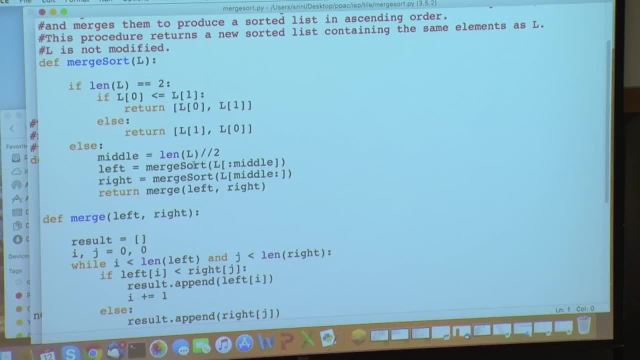 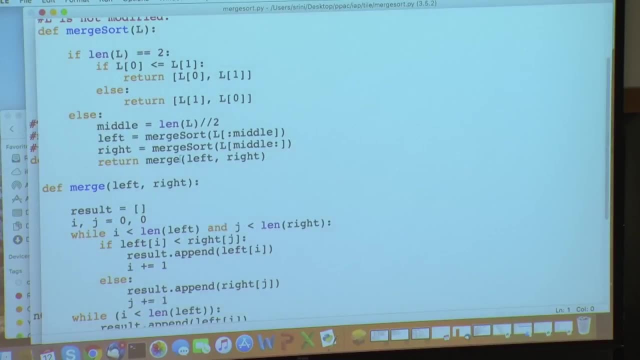 problems. In this case I'm using list splicing. So I'm using list splicing to get the first part of the list and the second part of the list And I'm just calling merge sort on those two lists, right, And then finally the workhorse in merge sort. 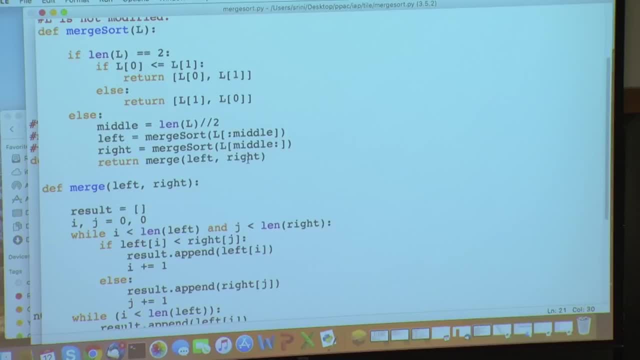 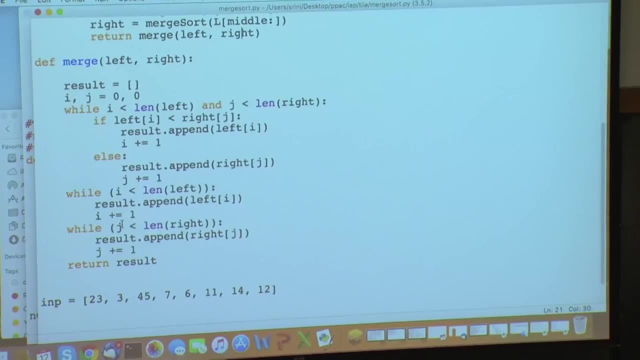 is the merge step, this two-finger thing that I just described to you. right, That is this merge thing. And this merge thing, as you can see, there's not a lot of code, But it's doing this movement and the comparisons. 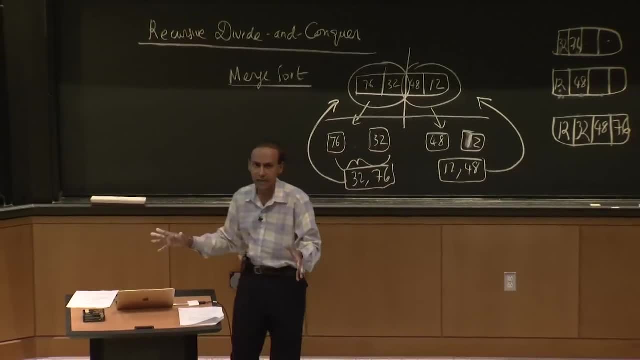 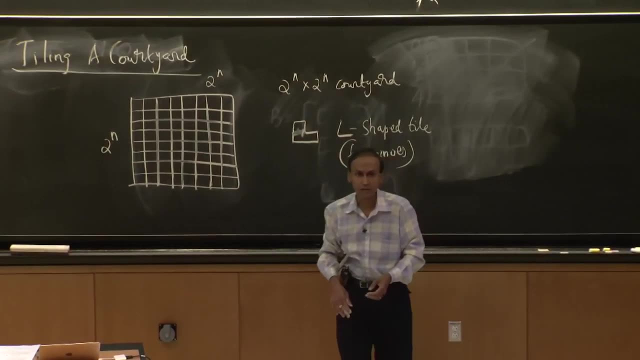 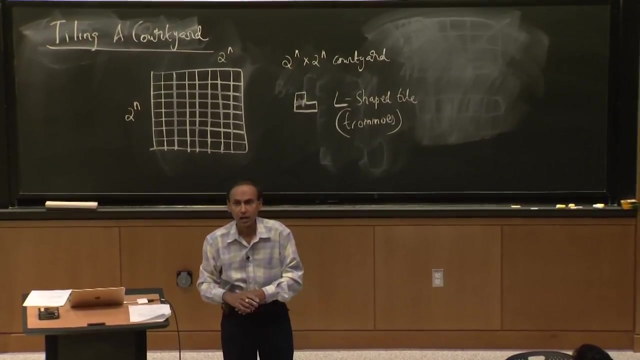 And that's essentially what you have there, all right. So, Given that context, let's go back to our tiling puzzle And let's talk about this tiling puzzle and how we could solve this tiling puzzle. all right, So you're going to break this courtyard up, clearly. 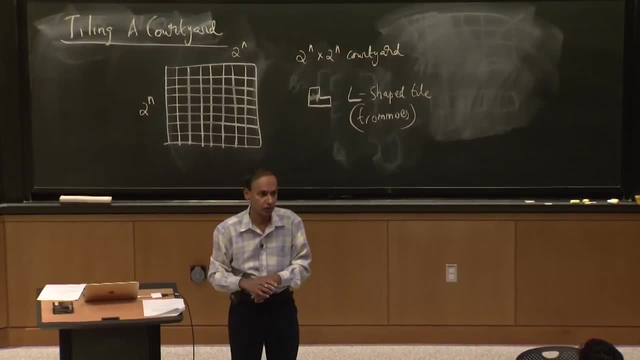 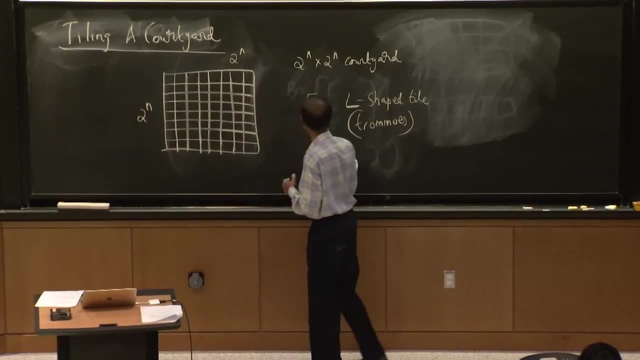 because that's really what I've been trying to tell you in terms of recursive divide and conquer. First question: look at this 2 raised to n and 2 raised to n and look at this tree tile. I'm going to ask you the question. 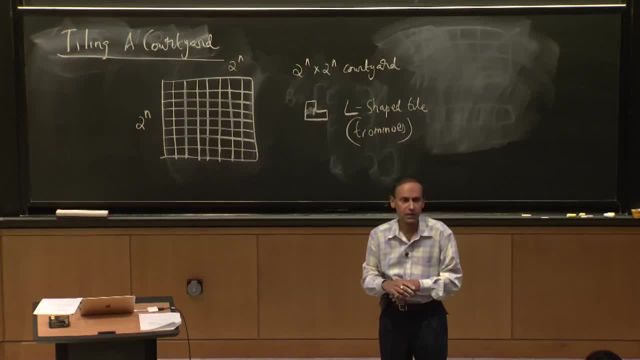 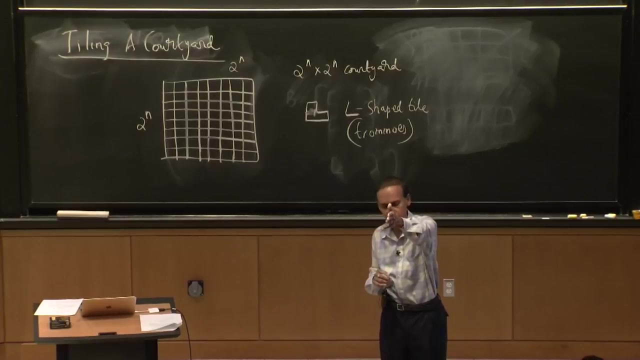 is there a solution that is, a perfect tiling with no overlapping tiles and no squares with holes in them? Is someone? Fadi had it, I'll hand it up first. Go for it. Well, I mean, if we look at the case, 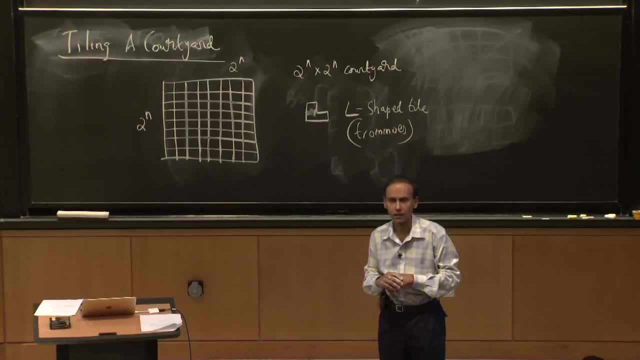 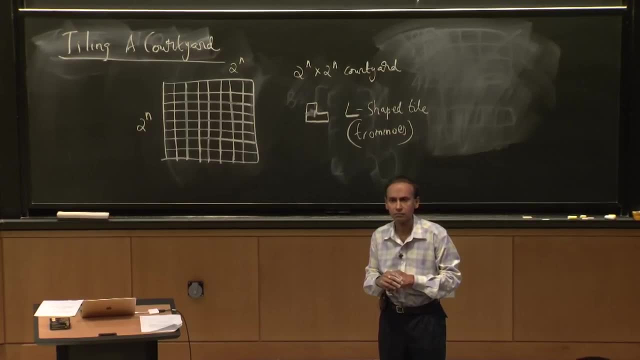 and it's equal to 1, and you have a 2 by 2 courtyard, then it's impossible to get back Right. You can't do that perfectly, But in the general case then we will have 2 to the 2n squares. 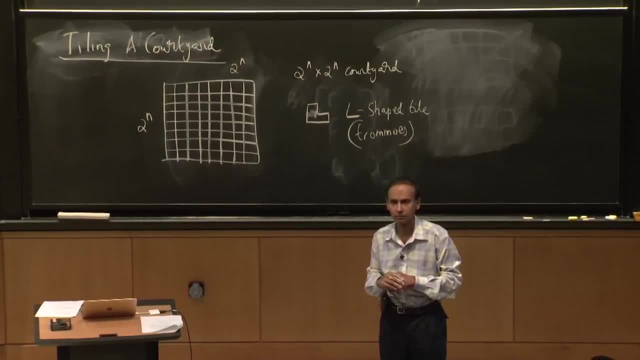 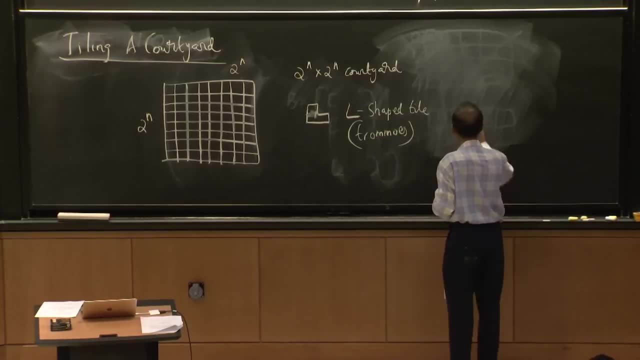 And every time we're adding 3,, 3,, 3.. So our number of tiles is going to be a multiple of 3. Right, So 2 to the 2n- and Josh probably had the same answer- 2 to the 2n is not a multiple of 3.. 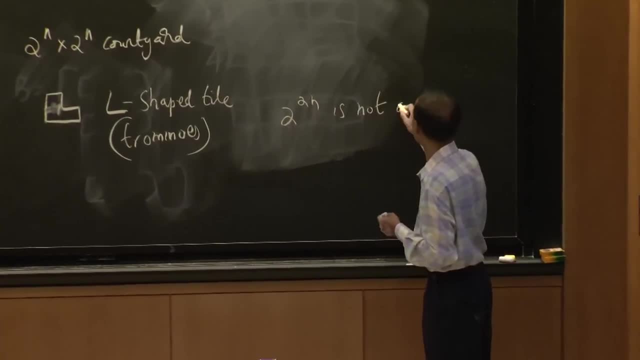 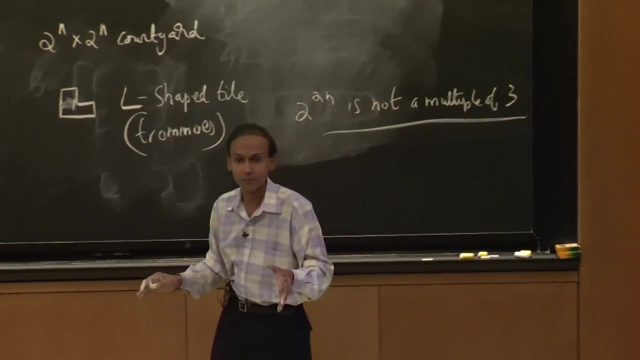 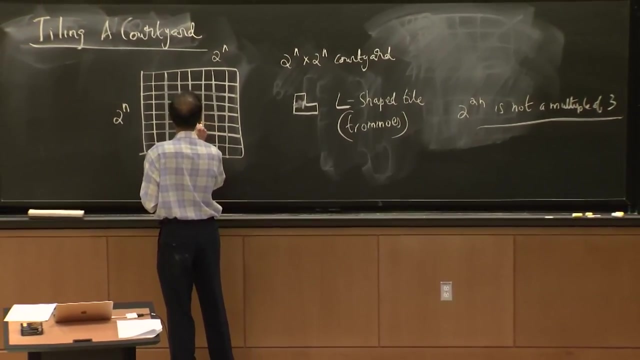 I mean, the only thing that divides it is 2, right. All right, So OK, So we're going to change the problem. All right, We're going to say that there's a statue of your favorite person that is going to be out here. 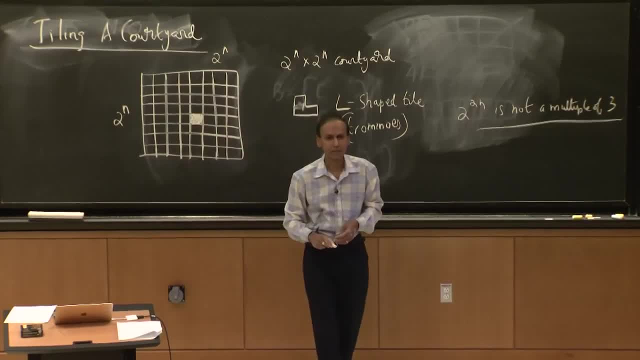 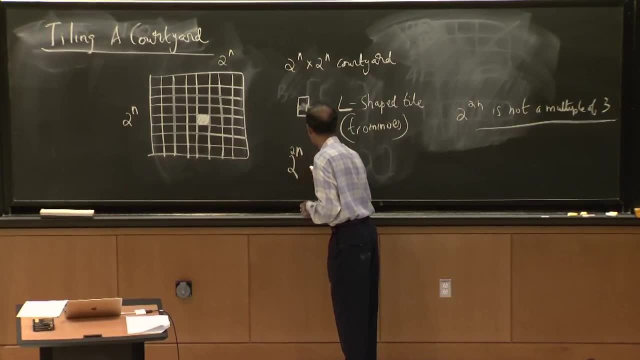 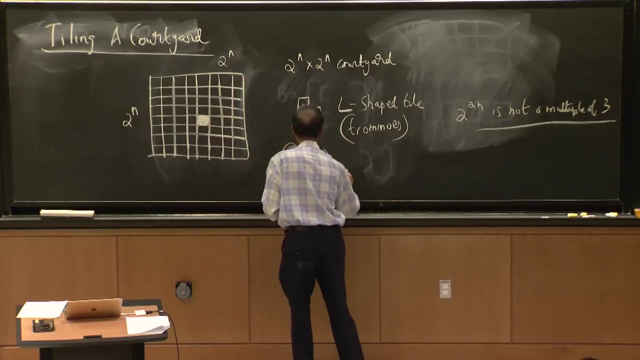 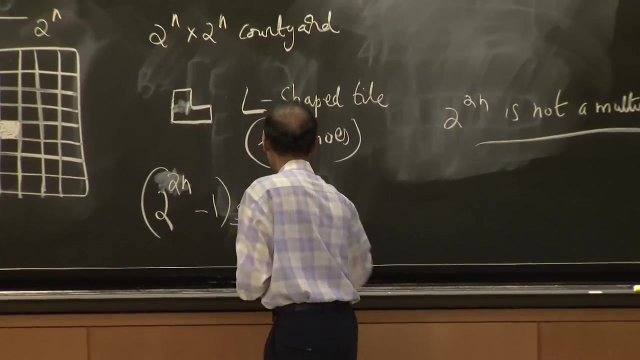 And so you don't need to tile that. OK, So now you have 2 raised to 2n minus 1.. Let me write that out properly: 2 raised to 2n minus 1. Squares Now can you do this for all n? 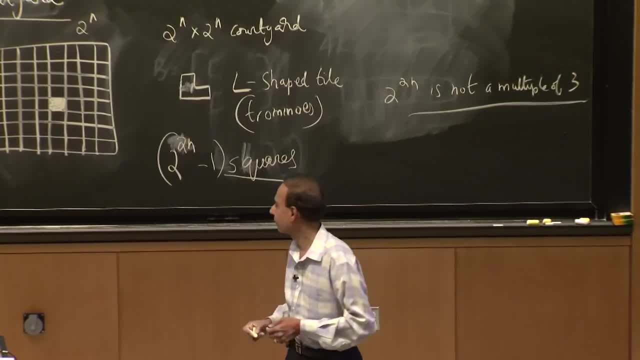 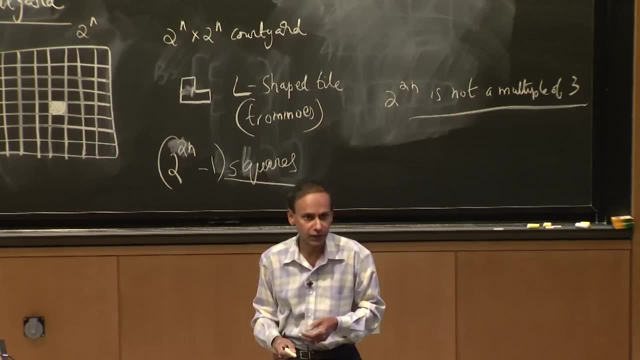 Clearly it works for n equals 1. Right, And then for n equals 2, you have what 2 raised to 4, which is 16 minus 1, 15. That seems to work, And then you get up to, I think, 80.. 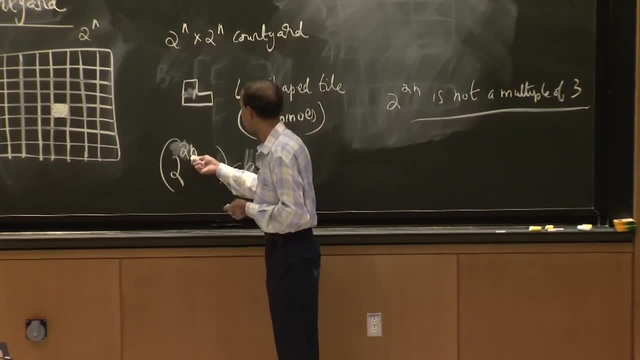 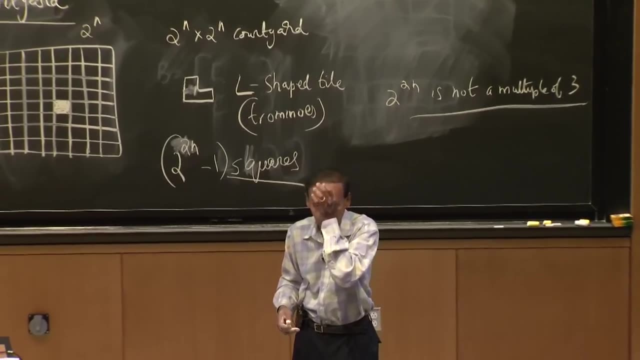 What is it? 2. 2. 2 raised to 6 would be 64. And so that would be 63. That works too In general. does it work? It does right. So it turns out if you think about it, if you have. 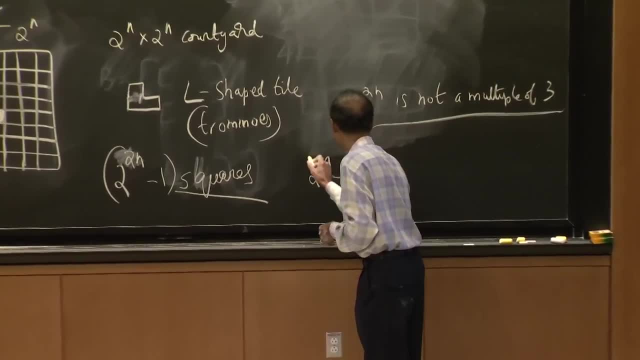 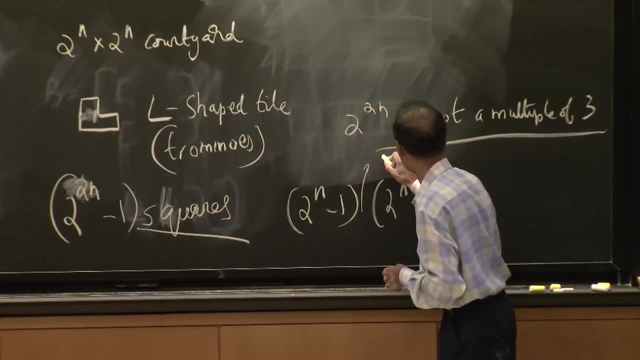 you can write this out as 2 raised to n minus 1 times 2 raised to n plus 1.. And in the middle there, pretend that there's 2 raised to n, So you have three consecutive numbers And when you do that you get 1.. 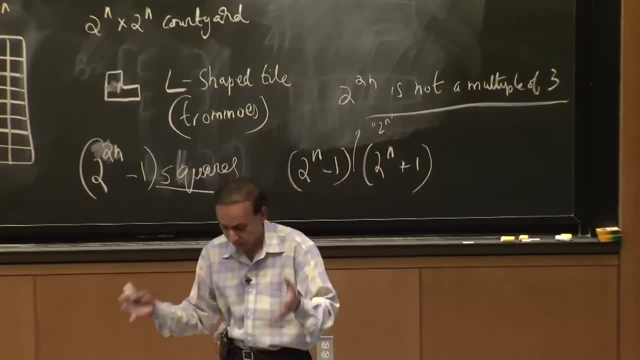 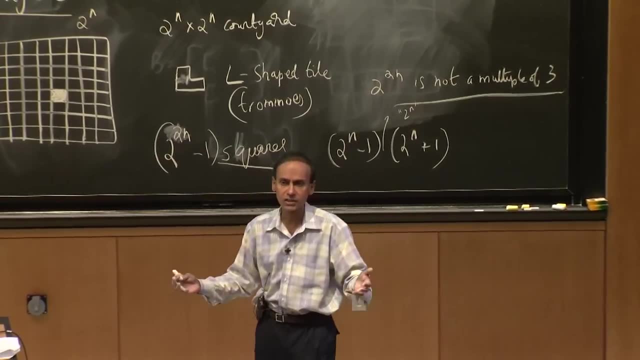 And then you multiply three consecutive numbers, And if they're consecutive, it doesn't matter what the numbers are. The product is always going to be a multiple of 3, right, Because one of those things is going to be a multiple of 3.. 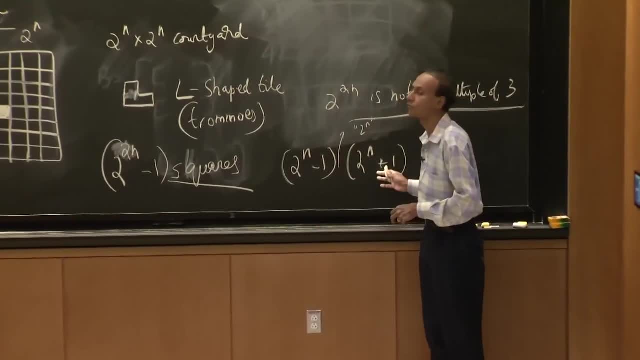 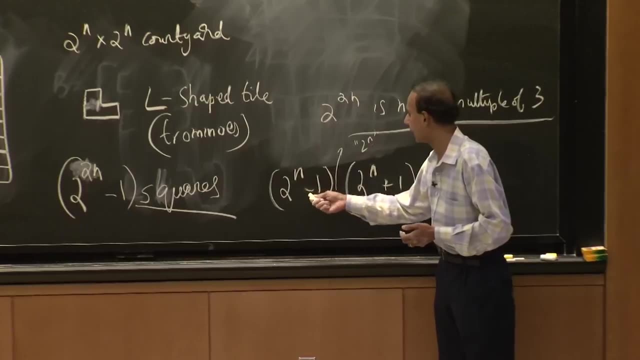 And you know that 2 raised to n is not a multiple of 3.. This is not a product of three consecutive numbers, But if it were, and you pretended that 2 raised to n was in here, either this one is a multiple of 3 or that one is a multiple of 3.. 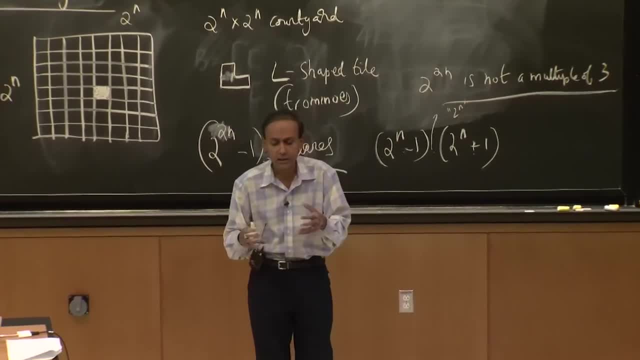 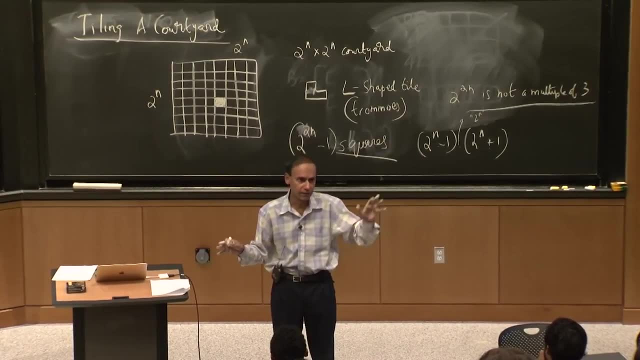 So this is good. So we know that there, At least from a standpoint of volume or surface area, if you will, that this is going to work, whereas the original problem didn't work from a surface area standpoint. All right, so it comes down to how. 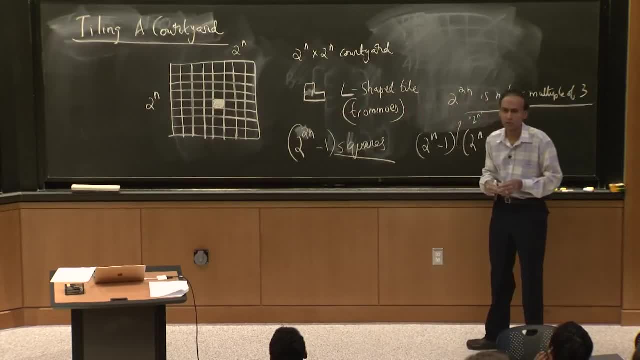 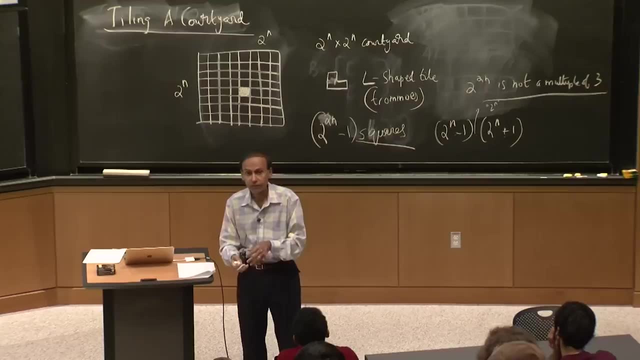 am I going to solve this problem using recursive divide and conquer And so I can break this up? And you want to have a similar feel to the merge sort where, when you got down to the base case of merge sort, you had this sort of trivial problem. 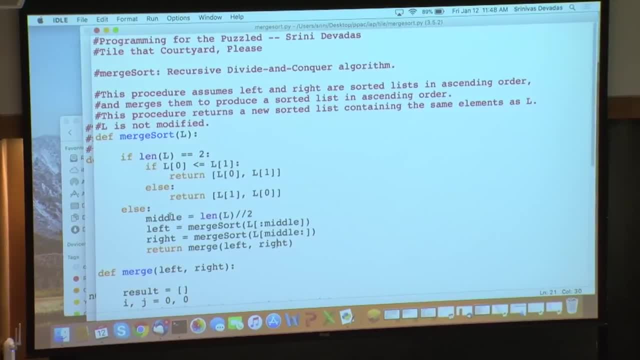 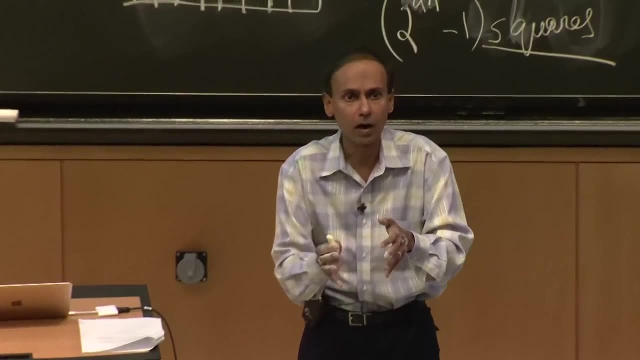 And you had a problem to solve. That's the beauty of divide and conquer. It becomes obvious when you have such a small problem, like one queen or I mean. that's technically not divide and conquer, but you do get to the smaller part. 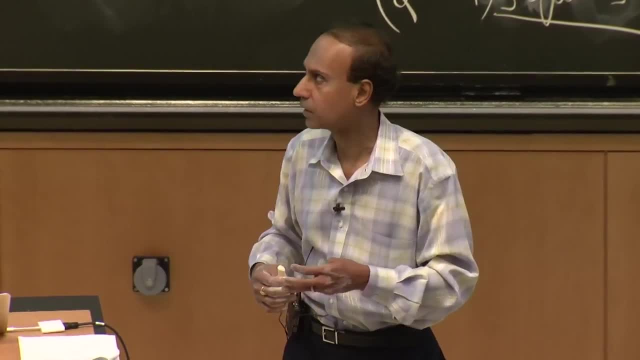 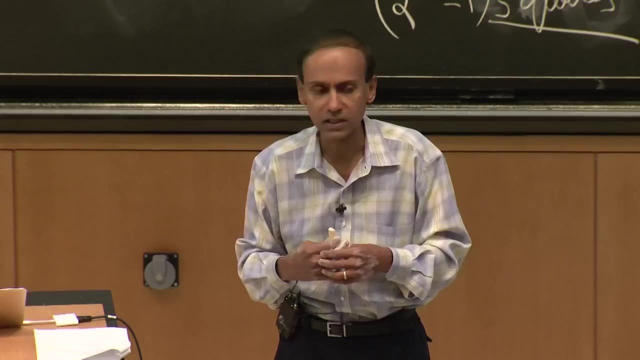 But clearly, in this case, this is a classic divide and conquer algorithm, merge, sort, And you can see that the first two or three lines of code are the trivial case of two elements that needed to be sorted. So let's go back and forget that. 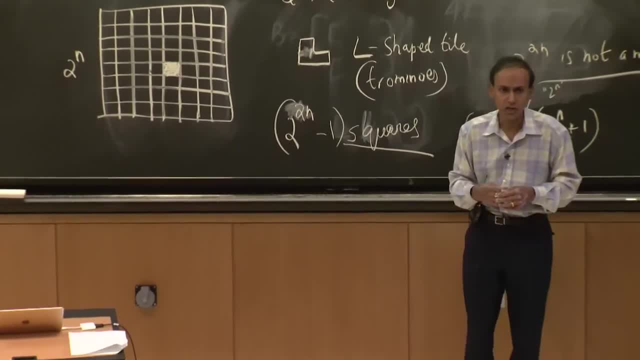 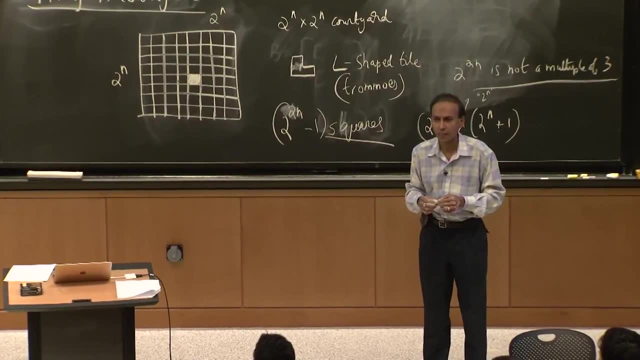 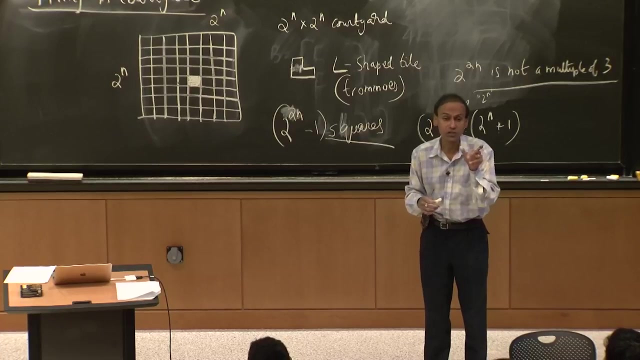 Let's look at this picture and think about how you'd break this up. right, How would I break this up? So think two dimensionally. Merge sort was a single dimension. OK, Think two dimensional. This is two dimensional, This is a two dimensional problem. 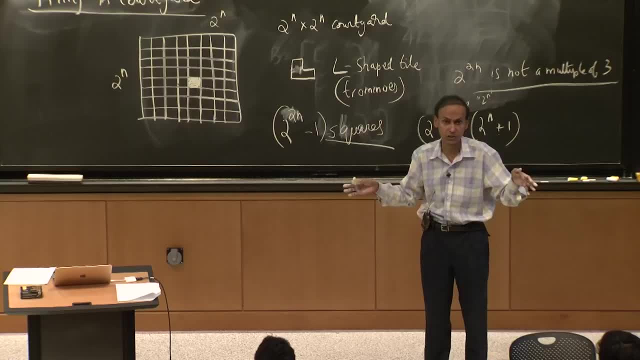 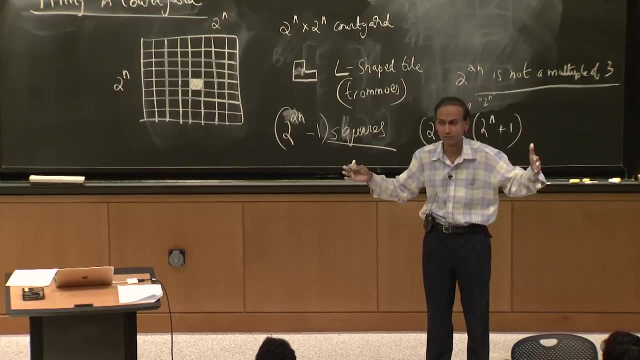 It's in that sense closer to n queens. But merge sort was simply a single dimension, right? All right, I see Kevin had his hand up. Kevin has his hand up, Someone else? All right, go ahead Kevin. 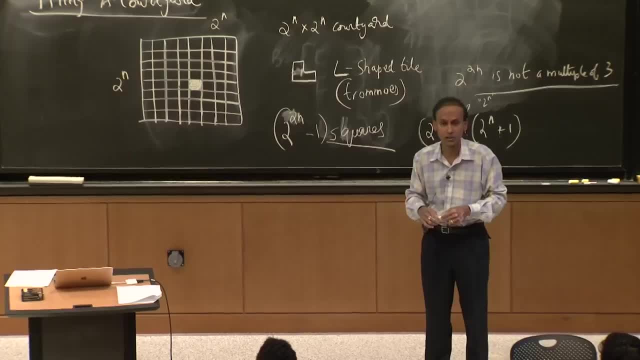 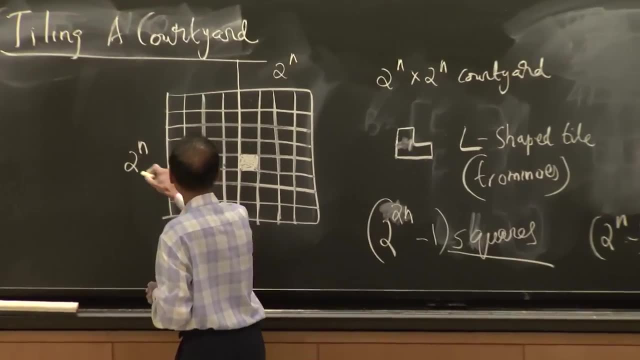 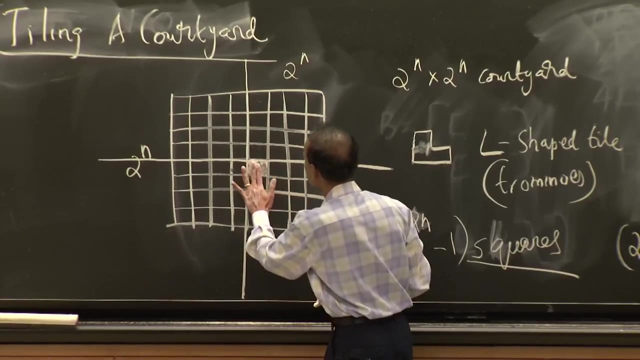 Could you keep cutting the square into quarters, Quarters, good, OK, yeah, All right, so let's do that. Let's do that. You're on the right track. right, And, by the way, this particular thing could be over there. 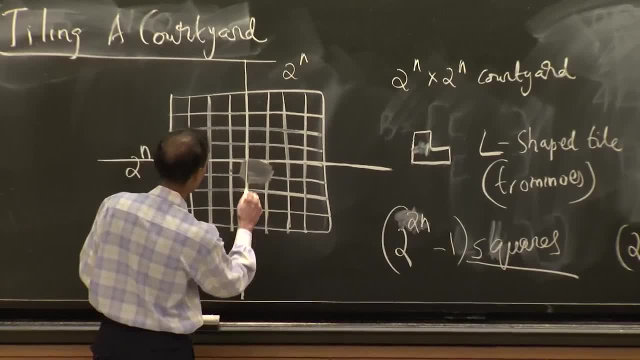 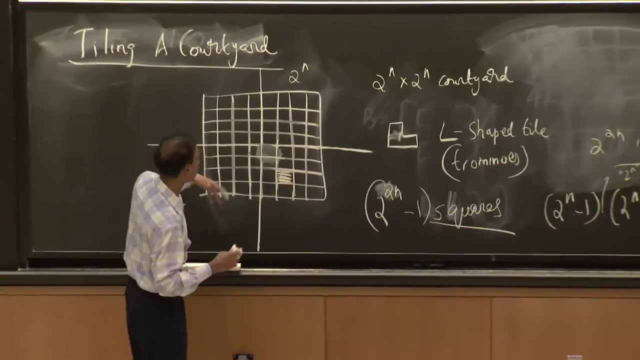 And I'll just do this just to make sure You can do this. Your algorithm needs to work regardless of where that statue is, So maybe the statue is over here, Maybe the statue is over there. There's only one statue that is covering one square. 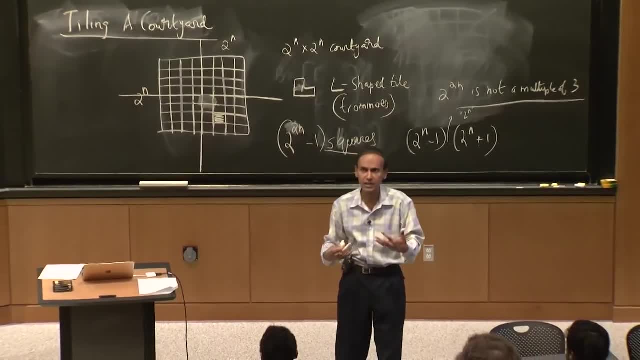 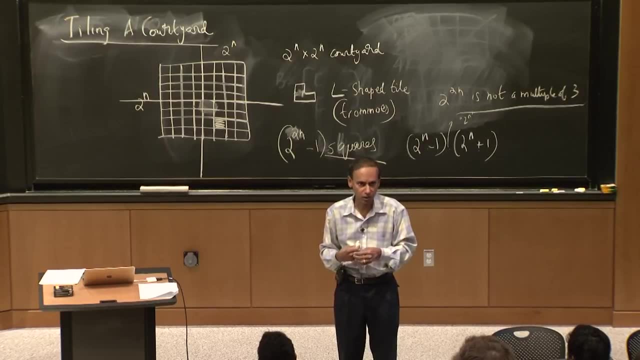 But it's not necessarily near the center. It could even be anywhere. You need a general purpose scheme that would work regardless of where the statue is, as long as it only occupies one square right. That's the only constraint we have, So you're on the right track, Kevin. 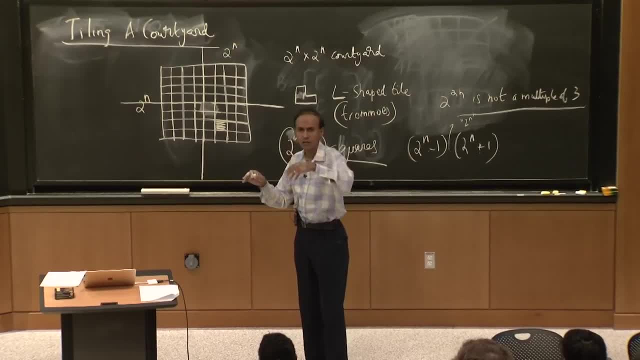 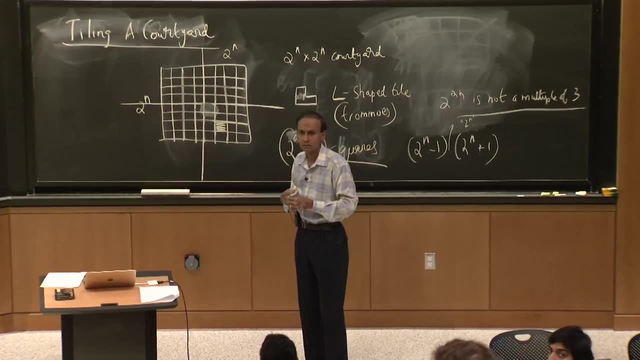 Someone else, or Fadi, you want to add to that? Yeah, So, like I mean, it's something that's similar to the merge sort. So if you divide into quarters and then we reach the base base and we tile that obviously. 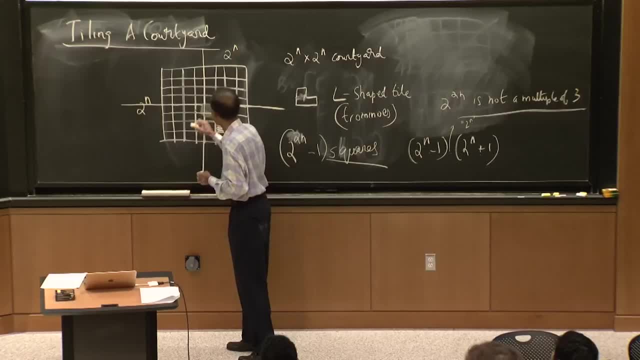 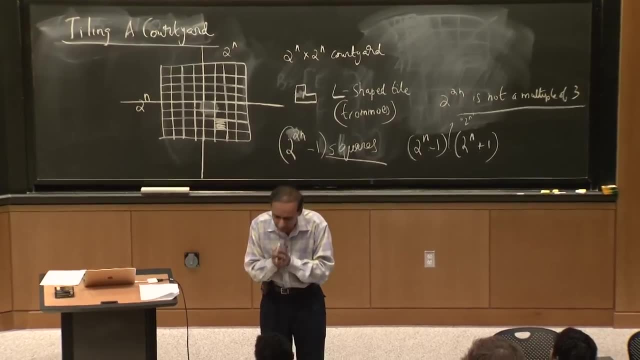 with a quick shape. Right, That's exactly right. Yeah, so there's one thing that's missing in what both you and Kevin have put up. The thing with merge sort was: I had exactly the same problem to solve. It was exactly the same problem. 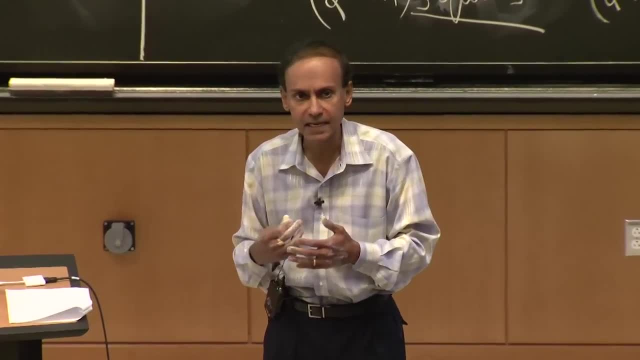 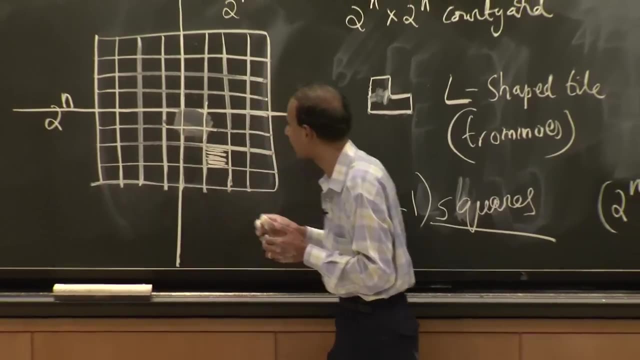 It was just smaller. I needed to sort the smaller array in a sense, And I had two of them and it was exactly the same problem. But when I split this up into four quarters, like you guys are suggesting, do I have exactly the same four? 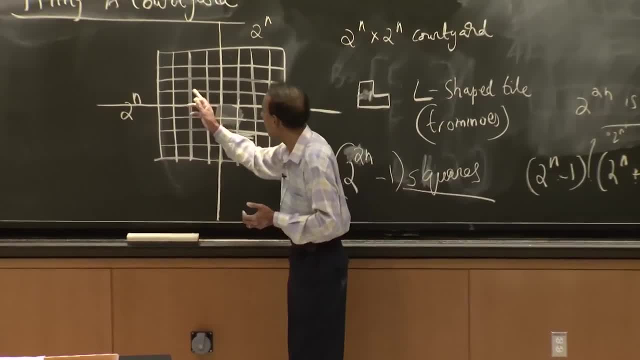 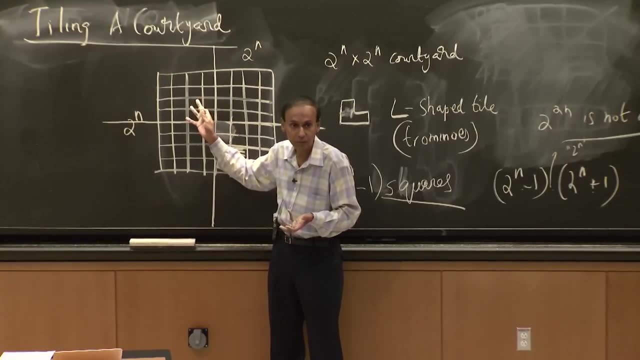 problems to solve. In fact, can I even solve this 16 problem with L-shaped tiles? I can, So at some level I have three problems that I can't solve and then a smaller problem that I don't quite know how to solve, other than maybe splitting it up even more. 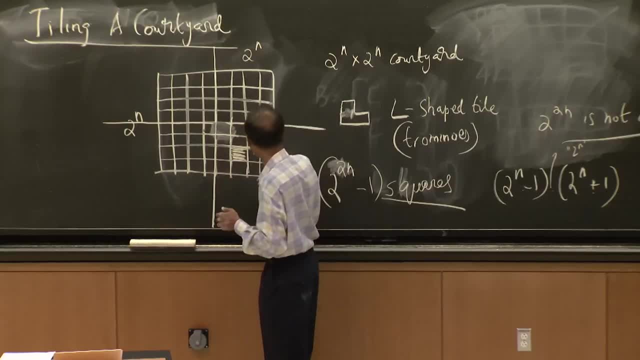 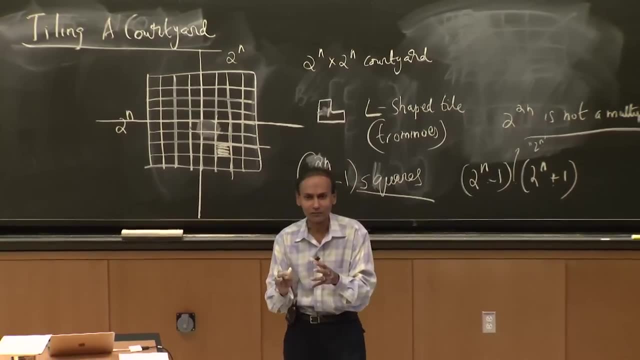 which is kind of interesting, which is good, right, But then the next time, if I go ahead and split that, then wonderful, I will find one problem, that's 2 by 2, that I can solve. right, But that doesn't solve my puzzle, OK. 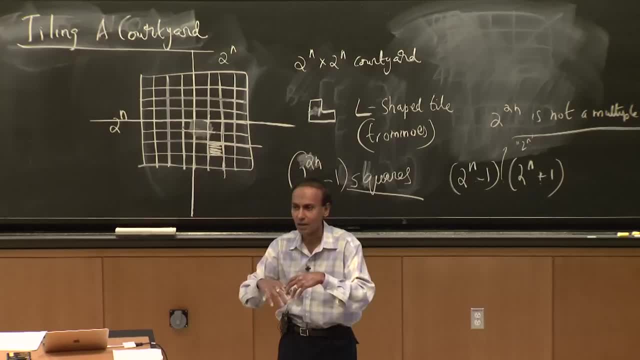 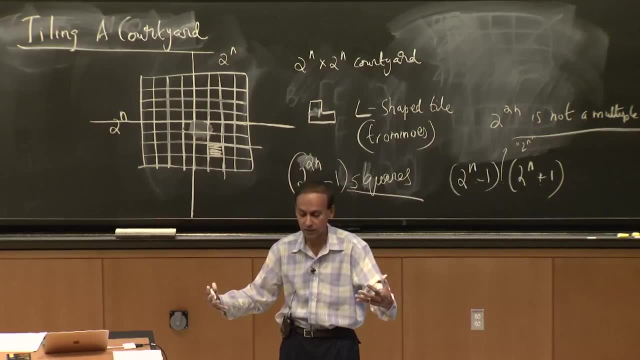 So I have to do one more thing in order to make this look like merge, sort or any recursive divide and conquer. One of the paradigms of recursive divide and conquer is: you're not creating new types of problems. You're creating the same type of problem except smaller. 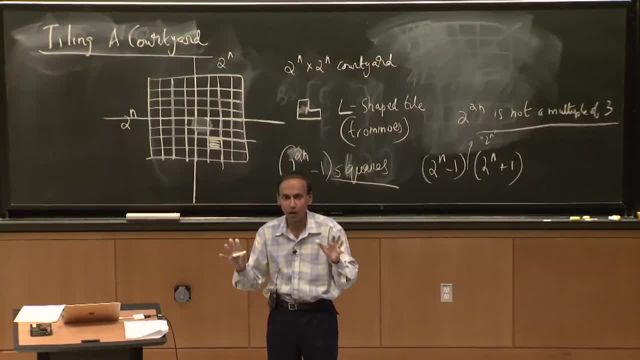 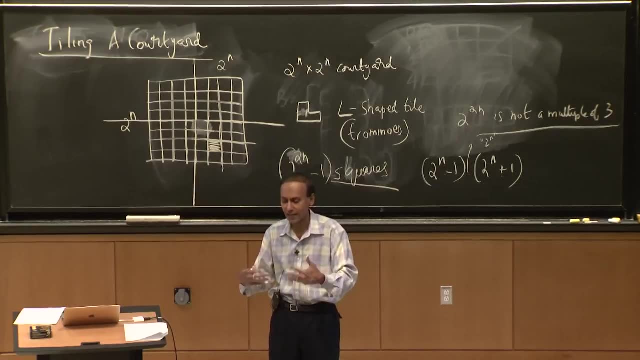 and therefore eventually easier. OK, So I have to do one more thing. all right, And this is an aha moment here that I'm hoping I don't want to take an answer yet, because I want you to think about it and perhaps arrive at it. 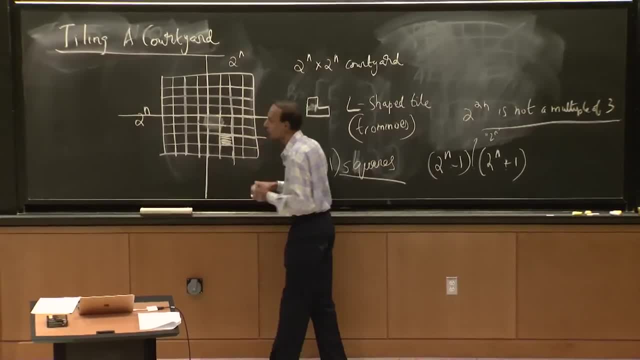 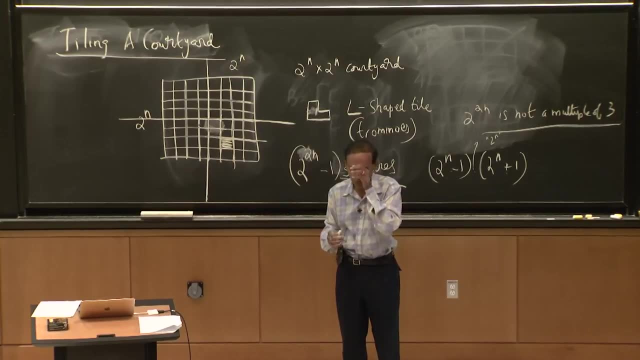 But it's one of those things where you're going to go, oh, if you don't know the answer, But it's worth spending another minute. OK, another minute each of you thinking about it, right? How am I going to set it up? so, these quarters, so all of this. 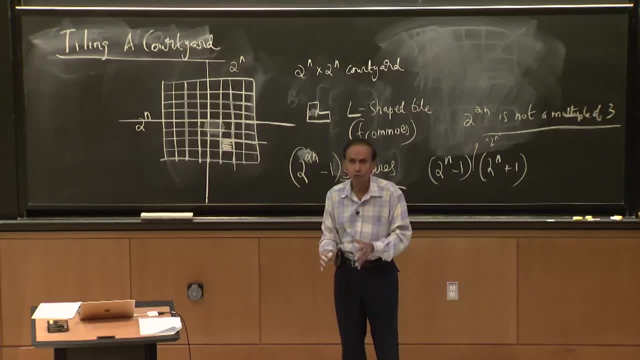 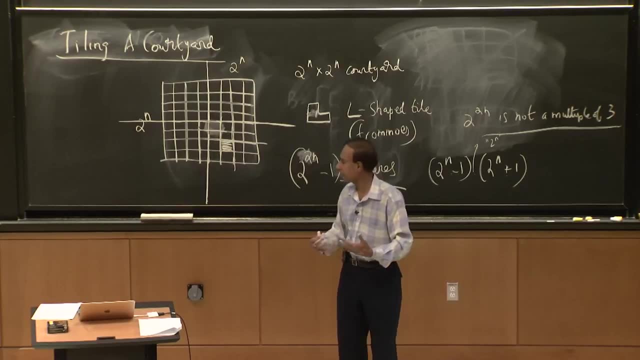 is good. We're going to split it up into quarters, But I want all four problems to look exactly the same, in the sense that they look. I mean, this obviously looks different from these other ones. There's a tile missing here, but there's. 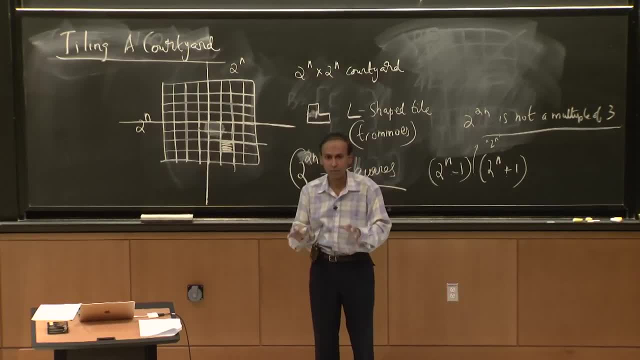 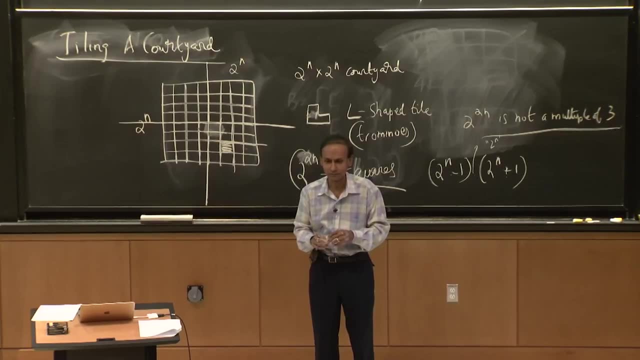 no tile missing over in the other three right. So how do I make all problems look the same? OK, I don't know if you know, but we need more. OK, I'll give you 30 more seconds and then I'll. 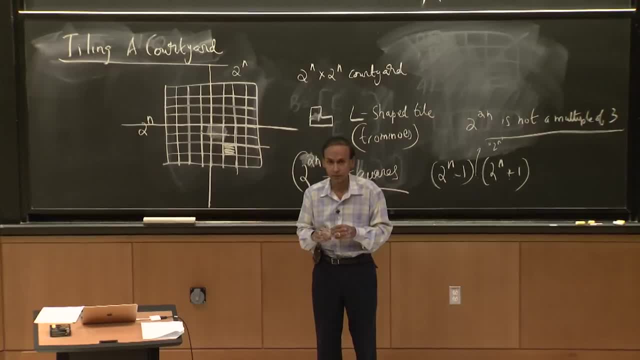 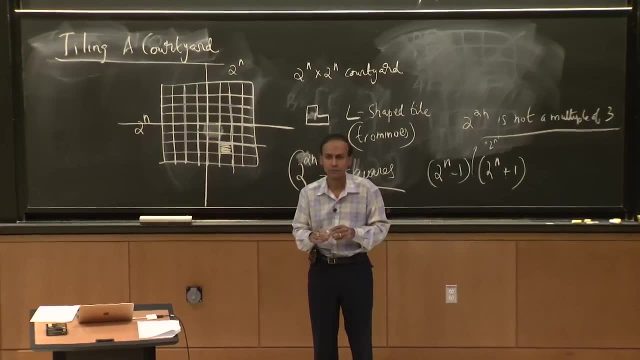 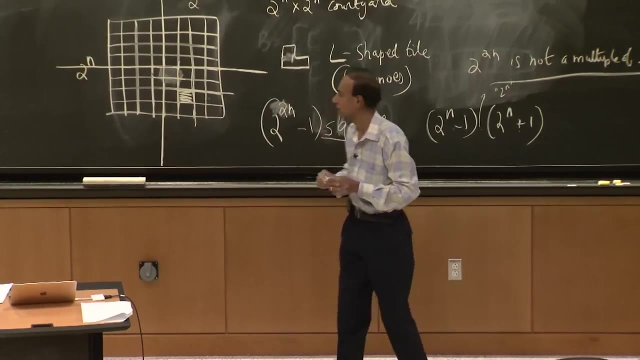 give you one more hint, all right. All right, the hint is: place one tile, Place one L-shaped tile. All right, yeah, go for it. Yeah, you know that, with those last four quarters, you know that the L-shape has to go around. 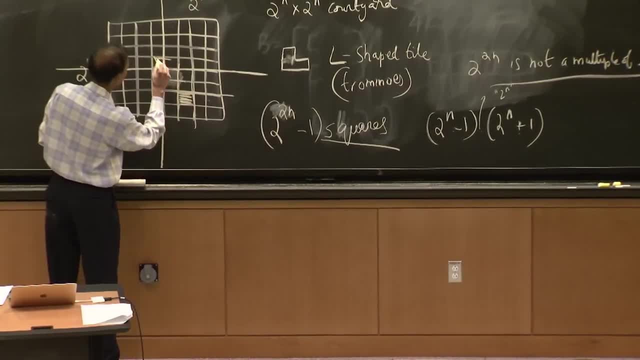 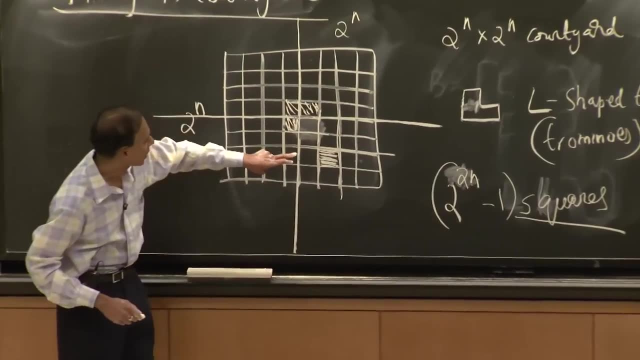 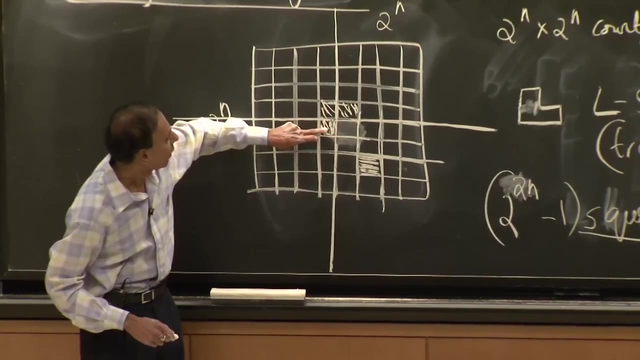 Yes, exactly. Yeah, that's right. So you set it up, so your tile. the reason I picked it up, picked this L-shape this way, is because this was the statue right, So I wanted to remove a tile from each. 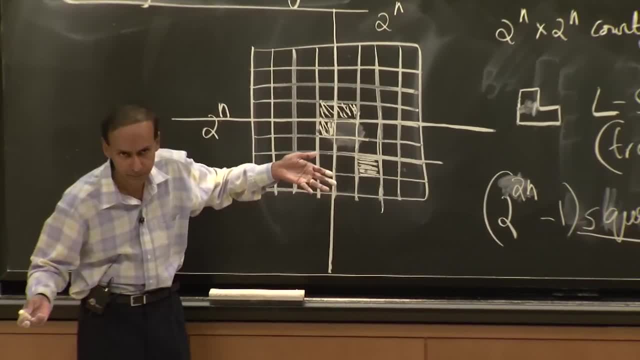 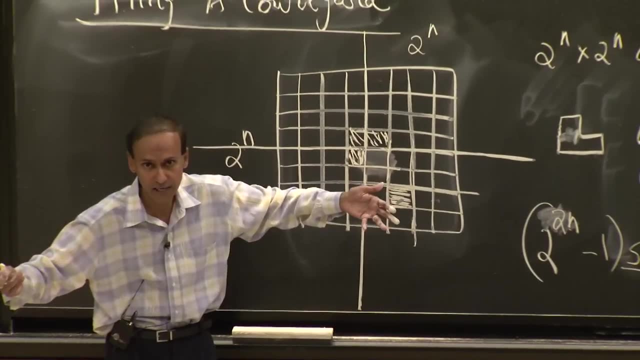 of the other three quarters. I'm sorry, remove a square right. A tile is L-shaped and so this was a missing square, which clearly was part of the specification of the problem. It has nothing to do with the tile, It's just a missing square because there's a statue on it. 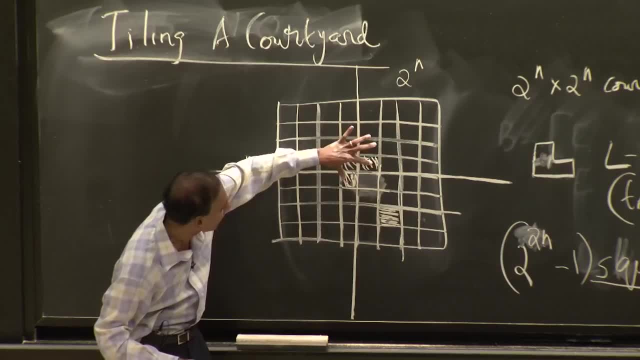 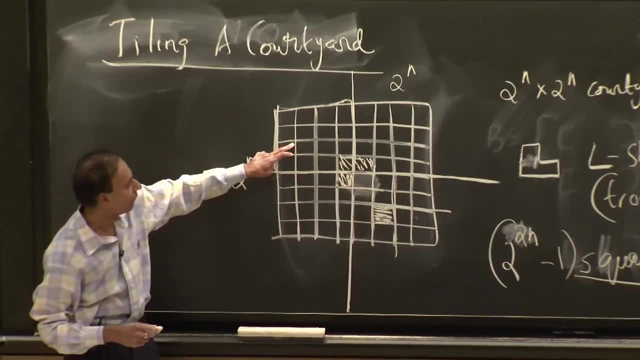 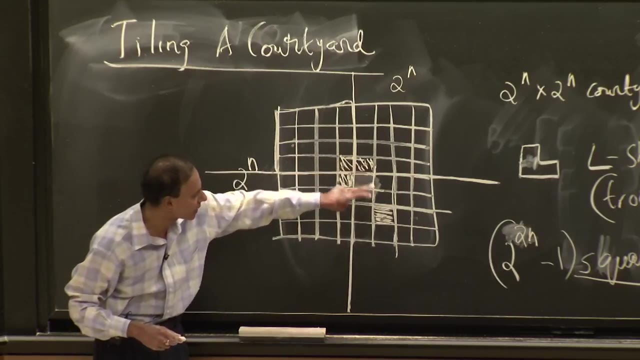 But what I could do is if I oriented the tile in this way. now I have- this being a smaller problem, which is 1 quarter of the size of the original problem, with one square missing. This one is one square missing. This one is one square missing. 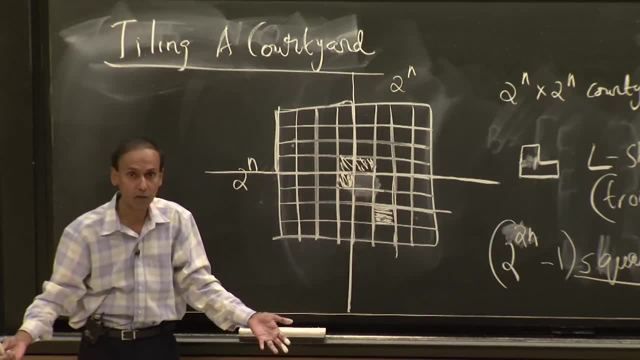 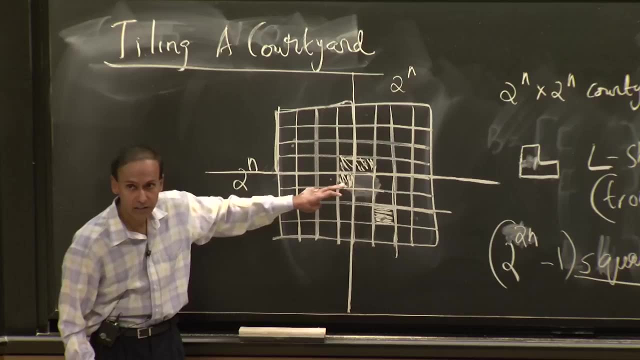 This one is one square missing. Now that makes all of the problems look the same. Now, of course, they're not exactly the same in the sense that the missing square is in a different position, But there's some generality that we need in our algorithm. 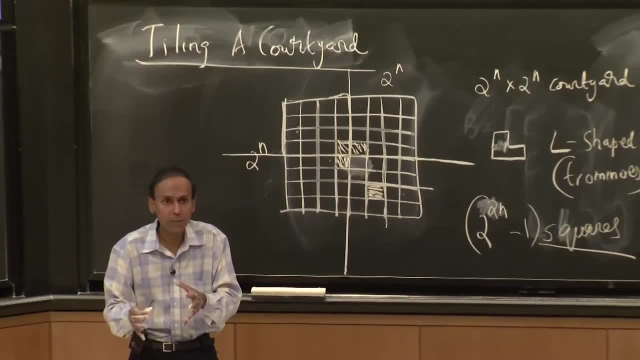 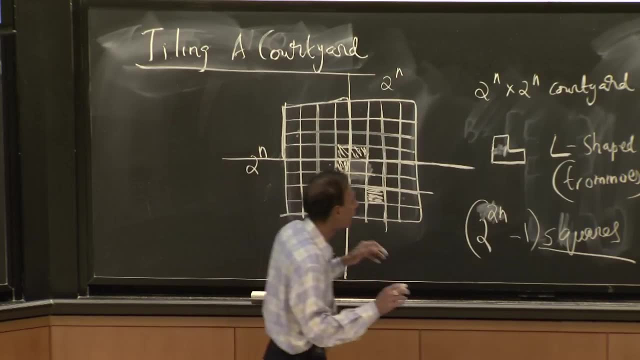 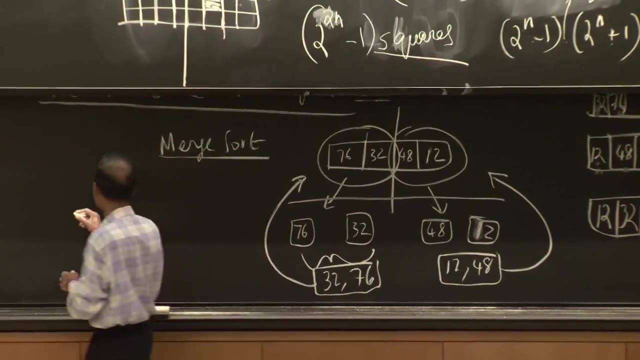 OK, That says that eventually, if I keep breaking this up in this fashion, I just need to orient my L-shaped tile in the appropriate way, right? So there's only four different ways that an L-shaped tile is going to be oriented, right? 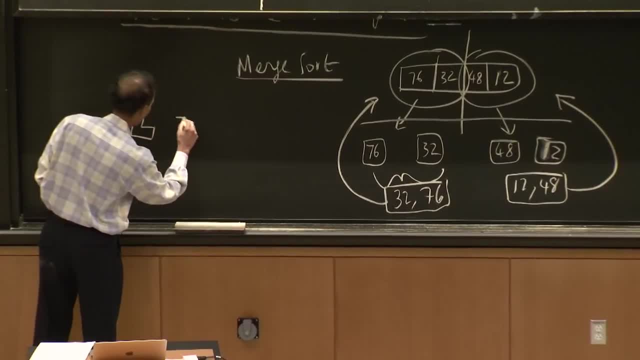 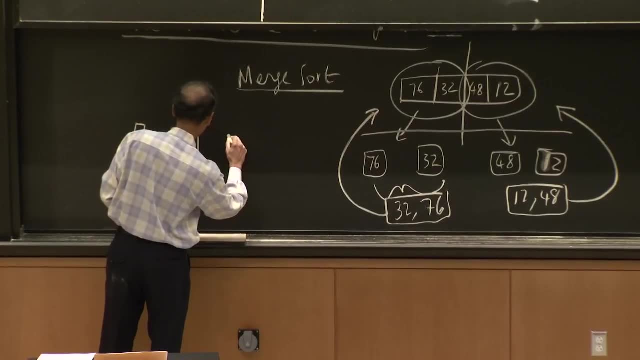 It could be oriented like this, and I won't draw all of them. It could be oriented like that, and it could also be that's the same. So what else is there? Oh, it could be flipped this way, right. 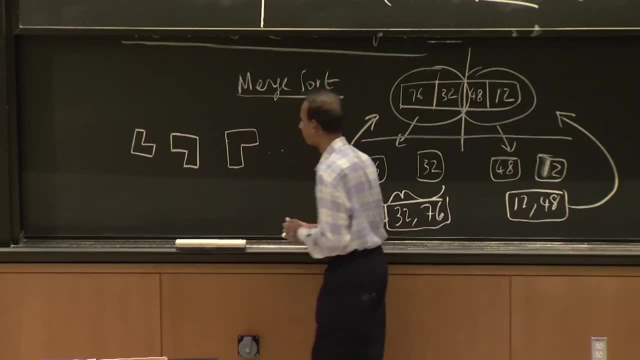 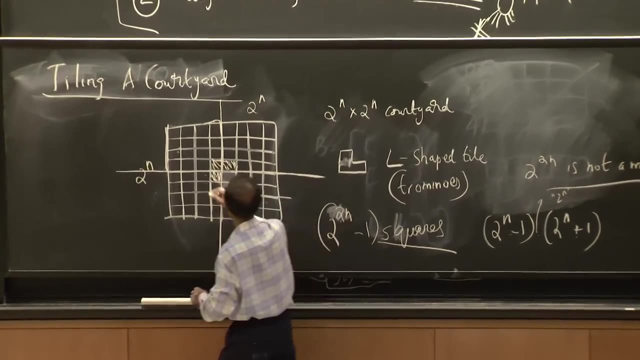 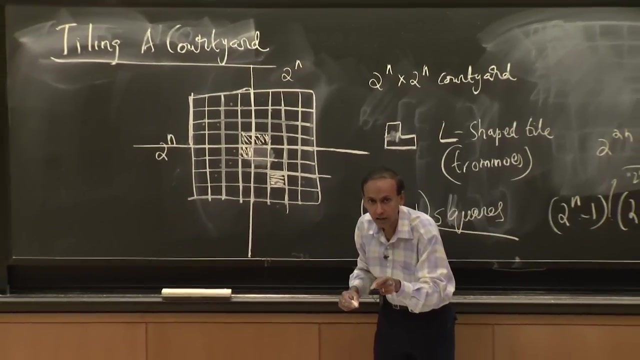 Yeah, Like that. and the fourth one. So that's what I did here. This one is what I put up there. And then, as I break this up, let's just say that now I'm going to make four recursive calls. I'm going to place one tile, one L-shaped tile. 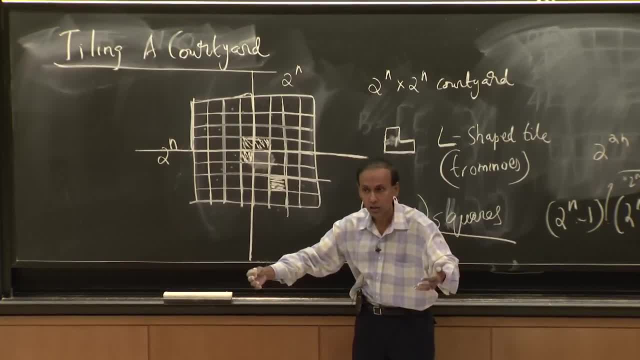 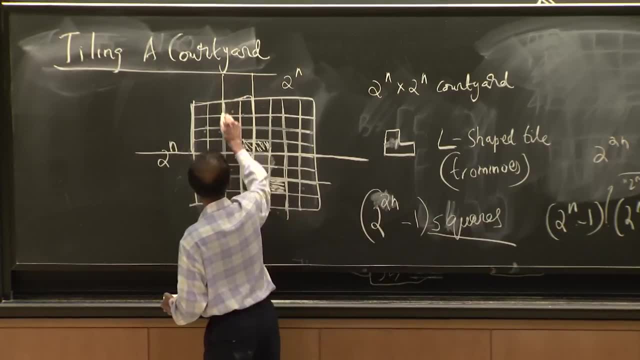 and I'm going to mark off these things and I'm going to make four recursive calls to basically myself, except that the arguments are different. right, It's the same thing, It's the same code, obviously. So when I go up here I go like that: 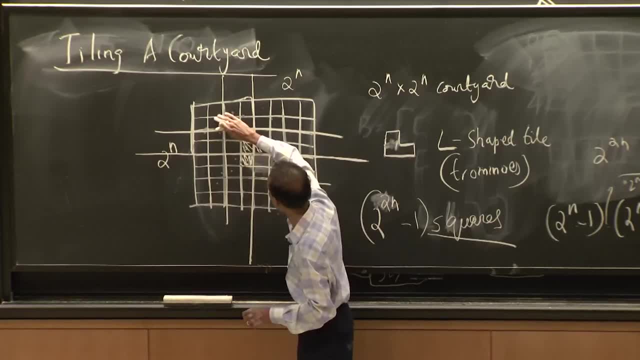 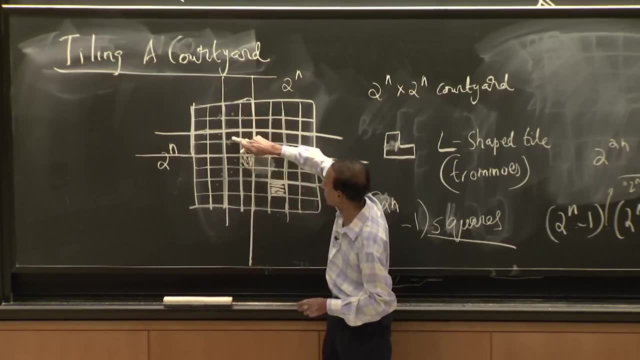 And hopefully this will become clear. We're going to do a tiling here. I'm going to go focus on the top left and I'm going to do this. What am I going to do with respect to this particular quarter of the courtyard? 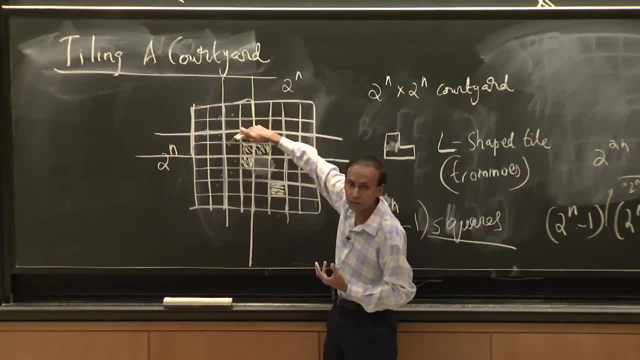 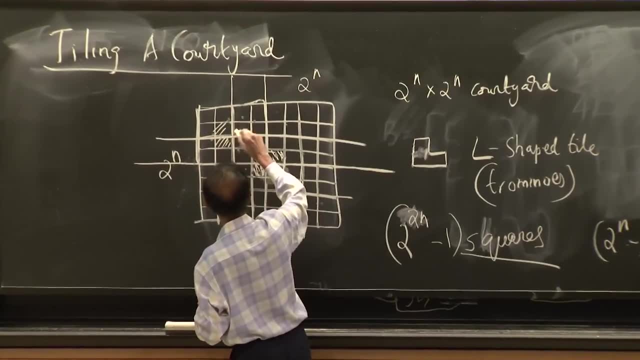 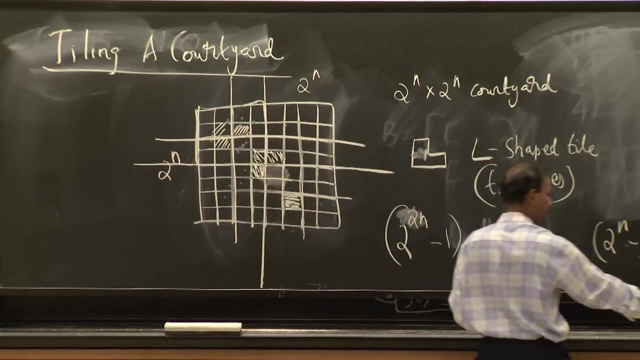 How am I going to orient the L-shaped tile for this one Point with your fingers? Exactly right, So it's the same as this. I'm going to go ahead and do that, OK, So now I have this problem, So I'm going to mark that with a different color. 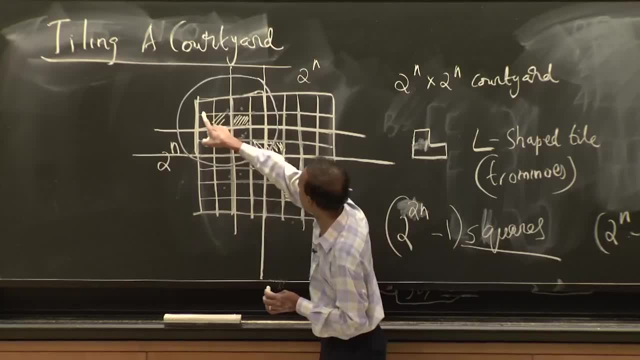 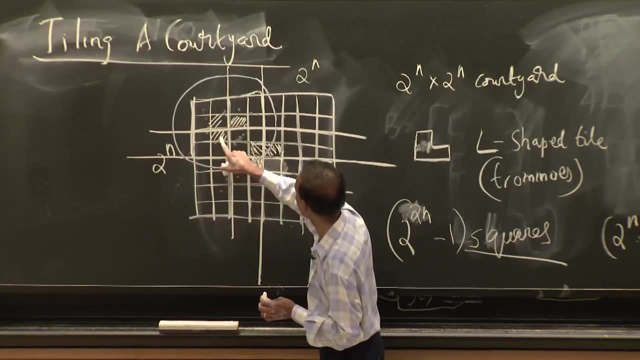 So I'm focused on this problem and I've done that break And now I'm good, because I have four 2 by 2 courtyards and each of these four has one square missing, in each of these four little 2 by 2 courtyards. 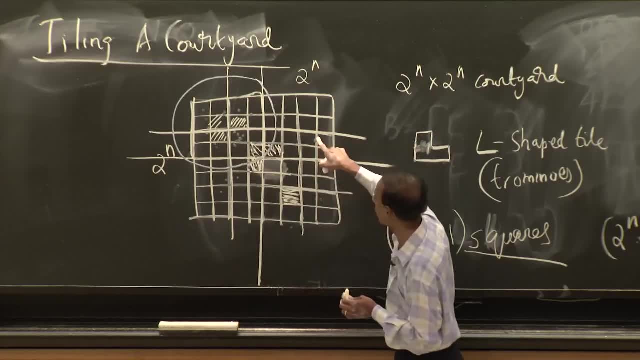 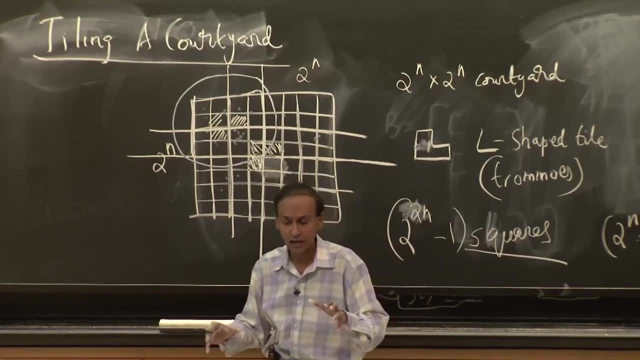 So clearly I can solve that And then, once I solve that, I can solve, I move on to this one and I move on to this one. whatever order you want, That's it, And so the code for this is from a control flow standpoint. 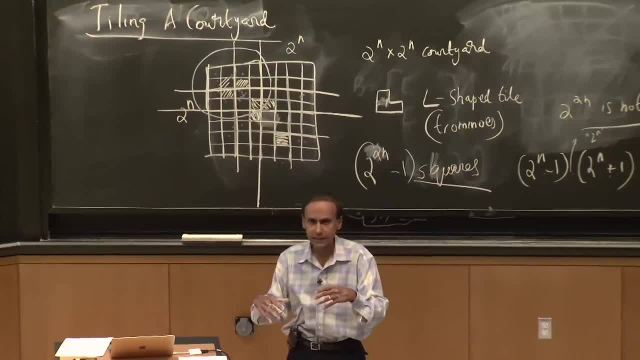 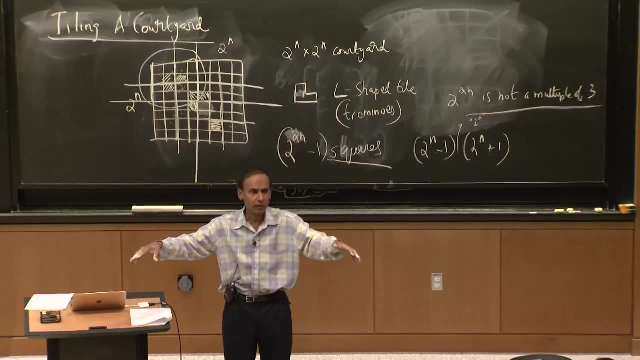 from a standpoint of the overall algorithm, it's extremely straightforward. It's almost exactly like merge sort, except that you have four-way recursion, because you end up getting it's two-dimensional and you end up getting quarters. And the only thing that's annoying about this code: 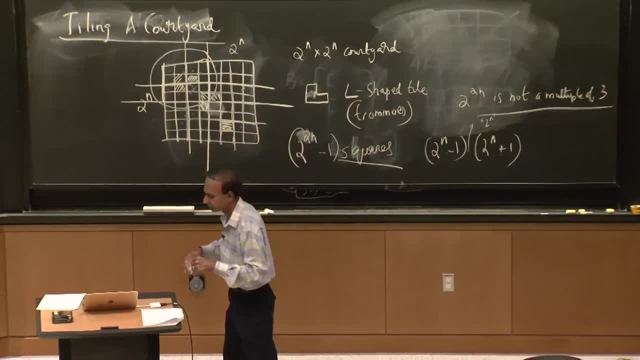 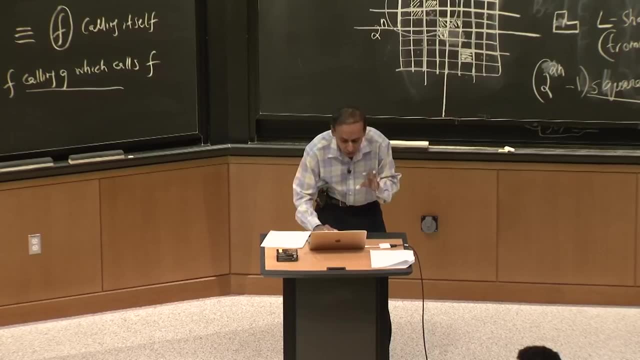 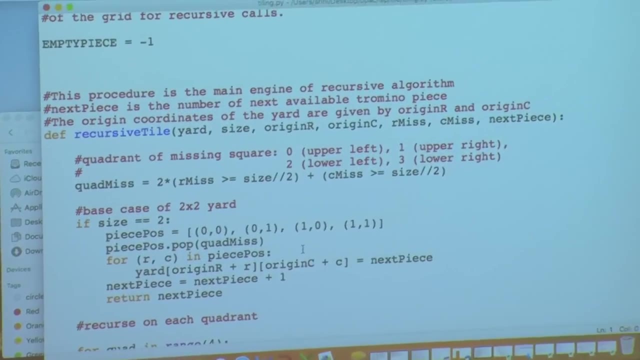 to write and also to understand, which you guys will love. I'll put this up and I'll show you what to look for is how you represent this such that you get all the values right. So you get an arbitrary square to begin with. that is missing. 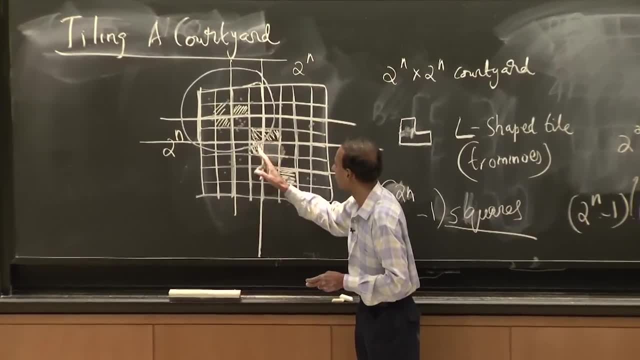 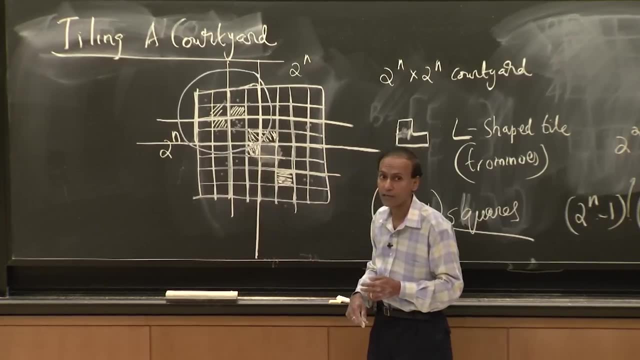 and then you have to go to the middle. That's clear. You're going to go to the middle of this courtyard and you're going to split it and you're going to decide which way this L shaped tile is oriented, And then you've got to do the splitting again. 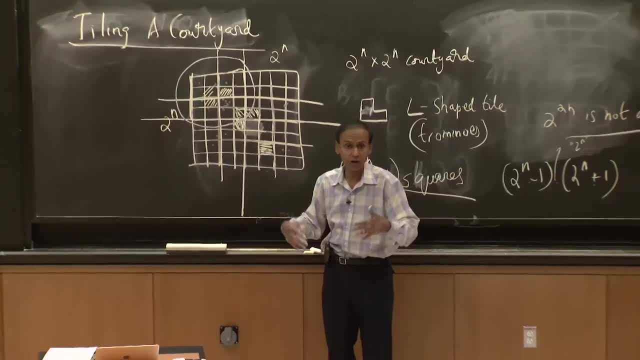 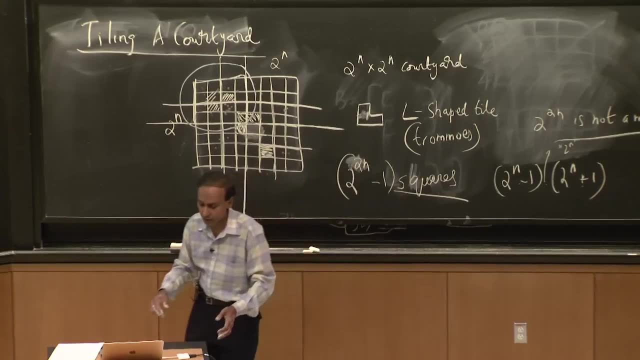 And so it's just bookkeeping. I mean, that's really what this is all about. It's not algorithmically interesting, It's just bookkeeping in terms of the orientation of these L shaped tiles. So if you look at the code and if you ignore, 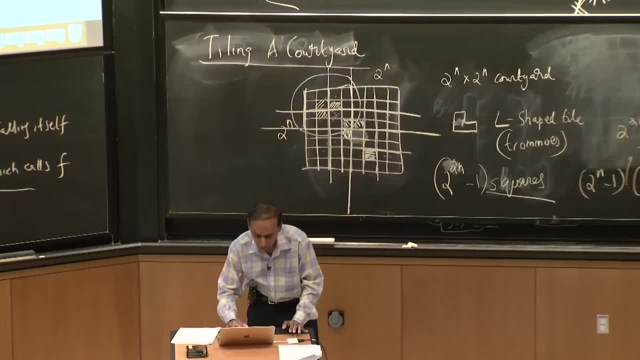 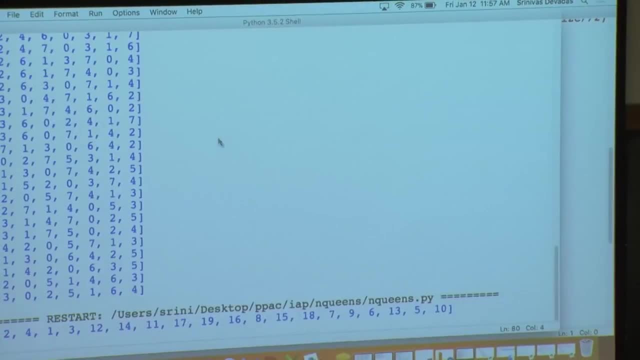 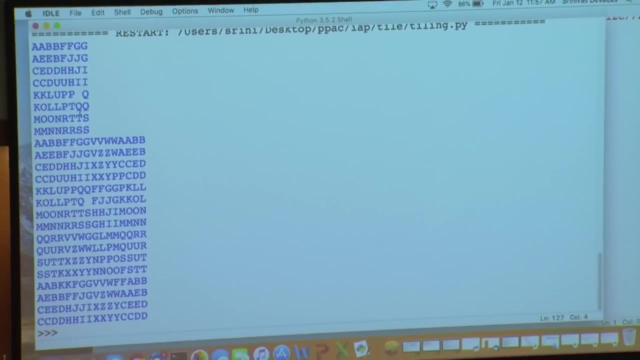 a bunch of these indices, of these different variables. let me show you. Well, first I'll show you what happens when you run the code. I'm running it for two different kinds of courtyards And I've used A through, I guess, something like S. 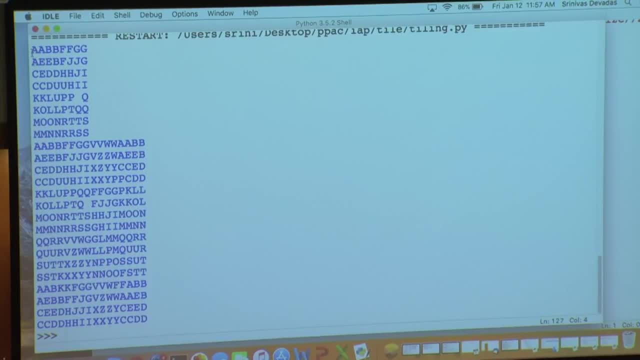 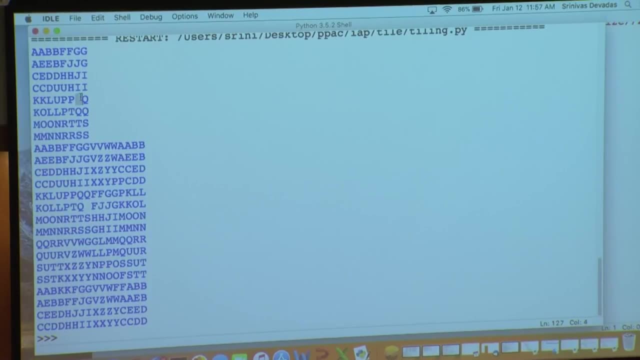 in this case to signify a tile. So you see AAA here. AAA is an L shaped tile, BBB is an L shaped tile, FFF is an L shaped tile, et cetera- The original specification of the problem. this is just simply an 8 by 8 problem. 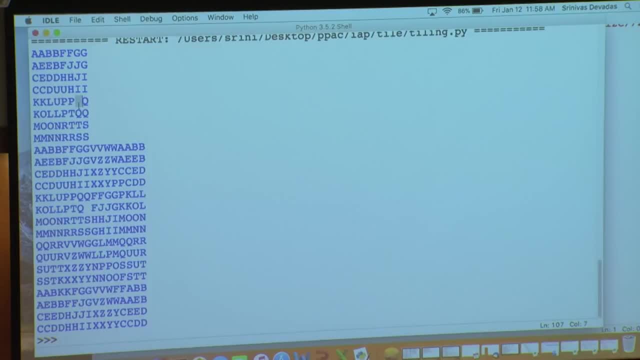 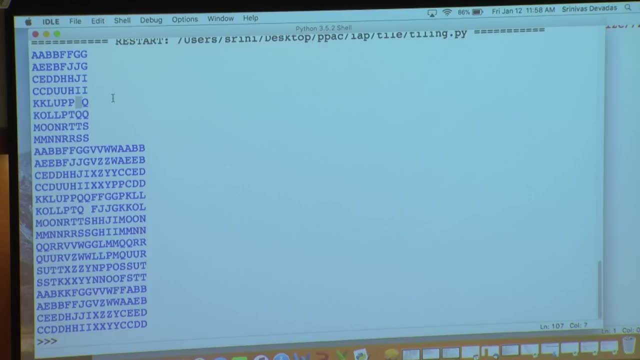 had this tile that you see here. that's a blank that I've covered up. that was missing, I'm sorry, the square missing. And then I broke this up into two or four, 4 by 4s, And then I went all the way up. 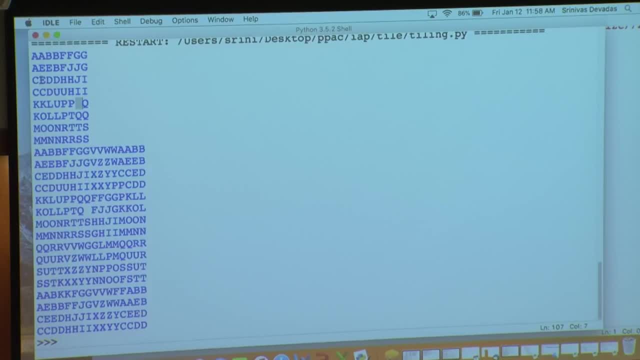 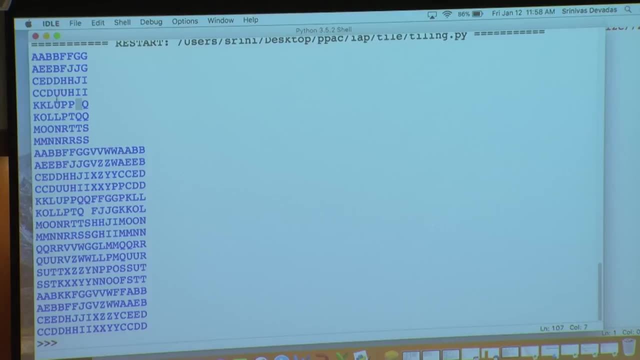 And then the first tile that I placed. I pretended to place this U tile over here. I could have placed it and then called it the A tile, But this is essentially what you think of the one in the center, exactly the way this is oriented. 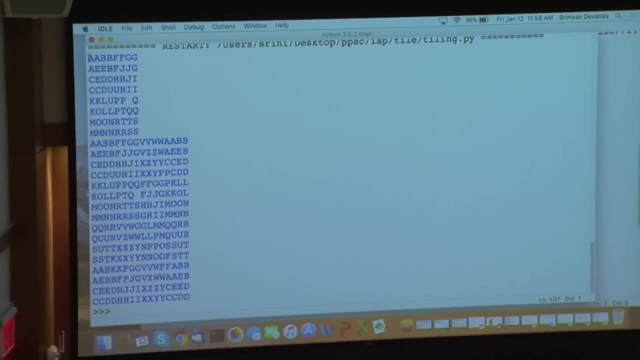 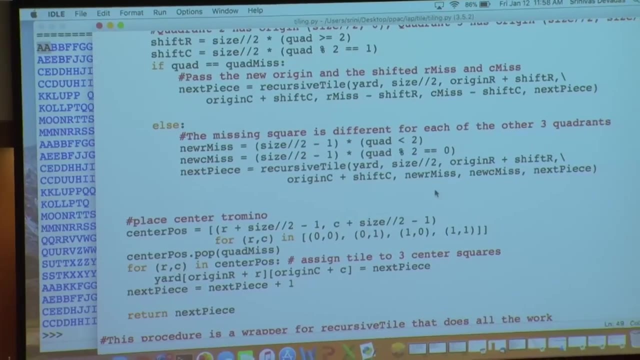 That's your U tile over here, And then you go all the way down And explicitly it's just the A tile that's placed first, And then the B tile, and so on and so forth. And if you take a look at the code, 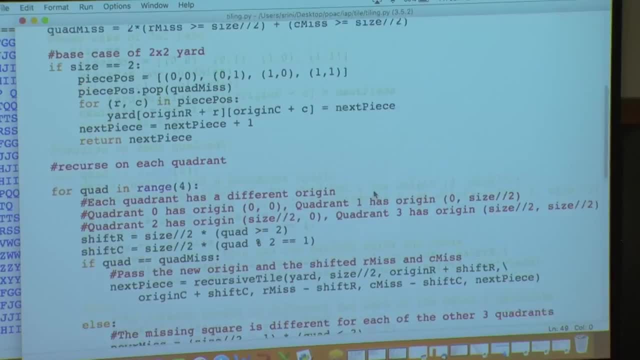 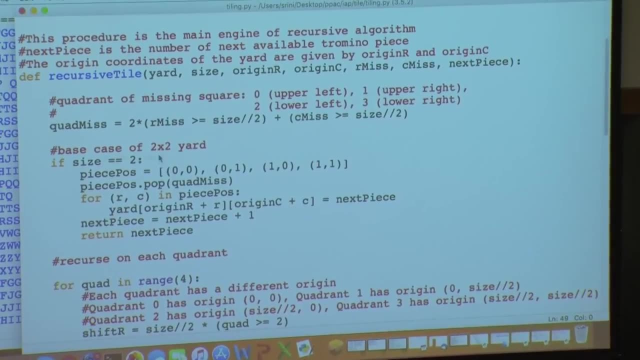 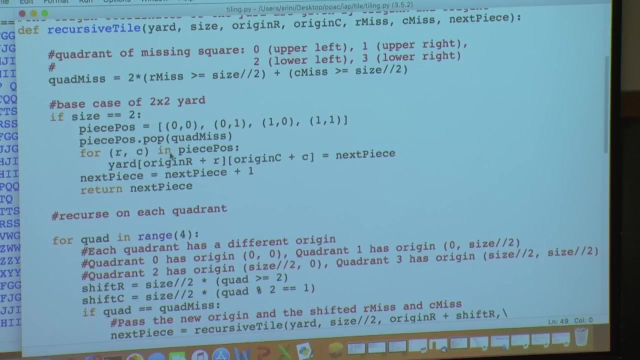 what's the best place to start. So this is the base case, Same thing as we've talked about before. You always need to have a base case. The base case is a 2 by 2.. And this code places one L shaped tile on a 2 by 2 yard. 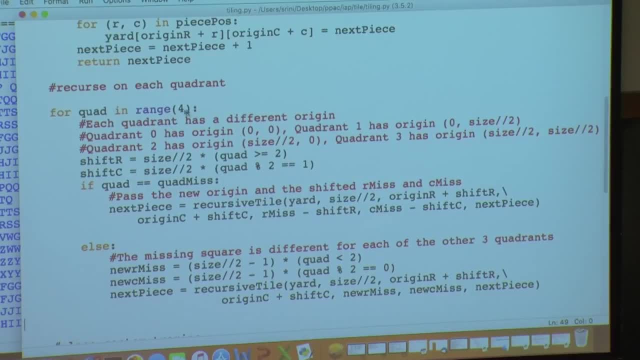 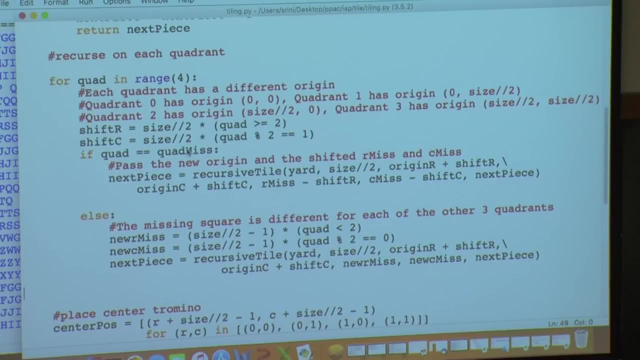 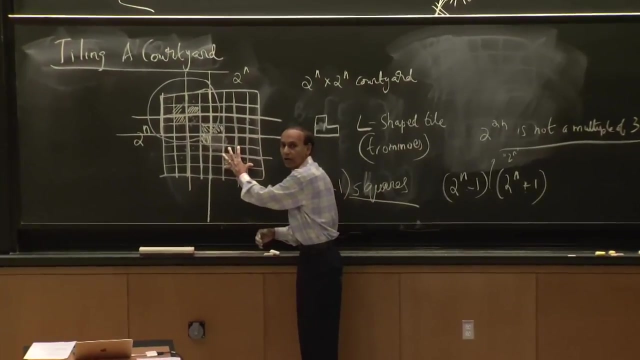 This is going to make four recursive calls, as you can see from range 4.. And there's two different kinds of recursive calls, in the sense that they're both calling recursive tile But the arguments to recursive tile are different for this recursive call.